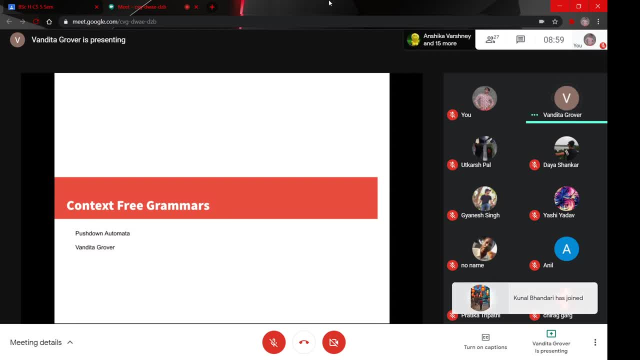 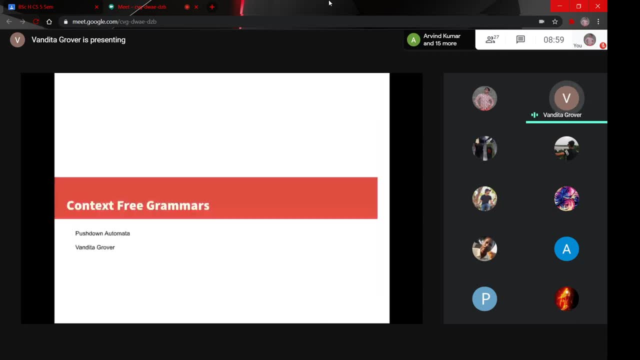 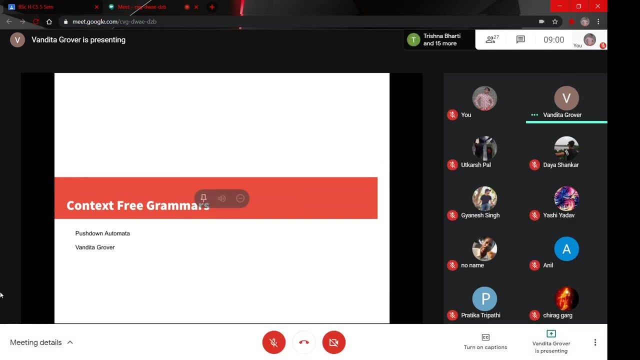 talking about the language acceptors for the context-free grammars. So do you know what a language acceptor is? Do you know what is a language acceptor? Anyone, Anyone who knows about the language acceptor? I have already told this, discussed this with you. What is a language acceptor? 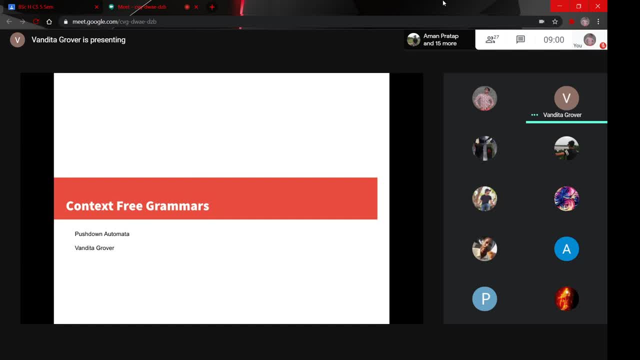 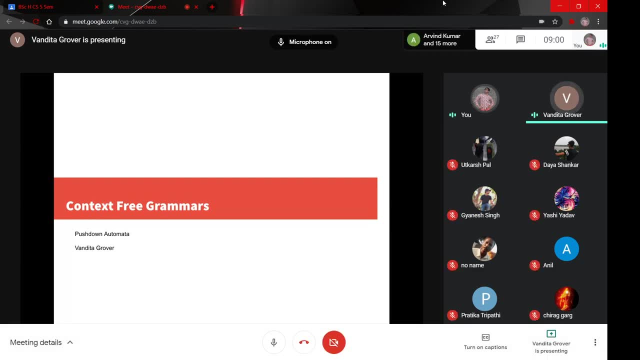 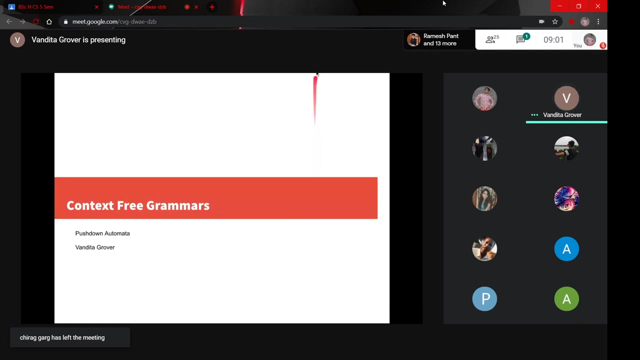 Can you hear me? Can you give me one example, Vibhu? Can you give me one example, Vibhu? Can you give me one example of a language acceptor? Can you give me one example of a language acceptor? okay, finite automata are examples of- and please don't put that in chat, i will have to. 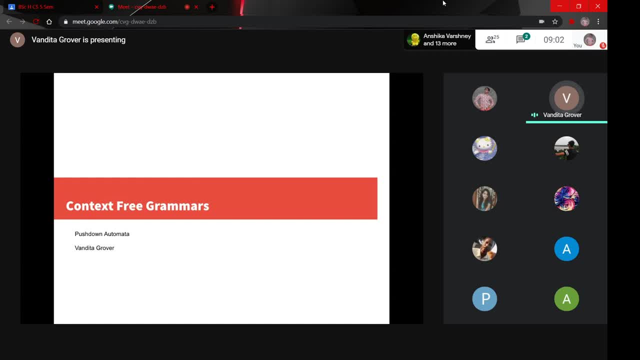 you know, keep on switching between my presentation and chat, so just kindly be. uh, can you think about me also? this is a finite automata, is also a kind of a language acceptor, because, uh, for regular grammars, regular grammars are accepted by finite automata, so it is a language acceptor. 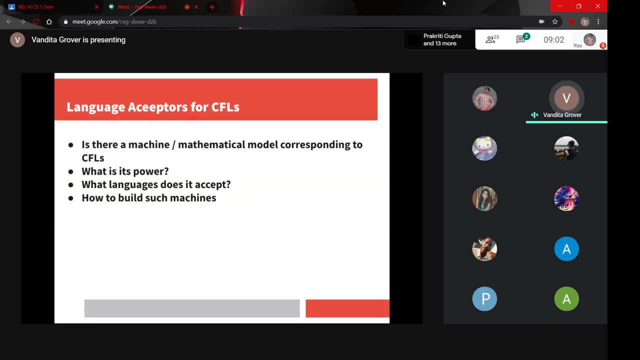 so now we have to find out whether there is a machine or a mathematical model. we said that machine is a mathematical model. finite automata was a mathematical model because we talked about finite number of states, we talked about a finite number of transitions, and over the input, uh, over. 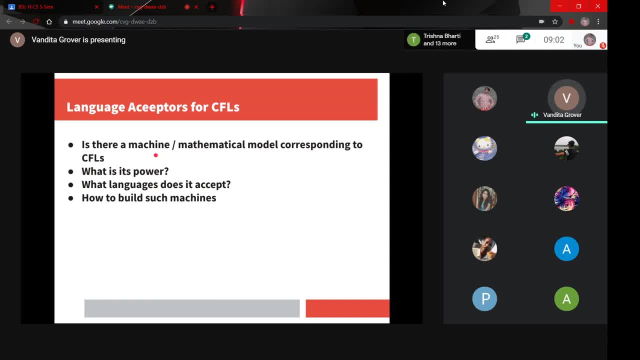 some input. what are the languages? uh, what is the language or what is the set of words it is accepting? so we defined a mathematical model. so is there any machine or mathematical model which corresponds to cfls or context-free languages? so, and what is the power of cfls if there is a machine which accepts the? 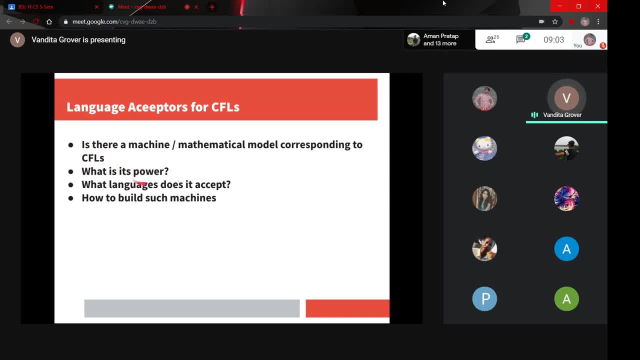 cfls if there exists, what is, how powerful it is, what kind of languages it can accept, for example? for example, a finite automata could accept only your regular languages. it could not accept, uh, your finite, your languages that are not regular. so can this, uh, uh, this machine accept languages which is, uh, which are? 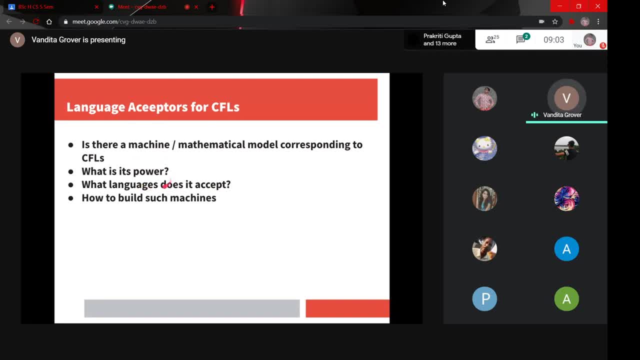 which are not regular, which are so regular like regular except, regular except, and uh, how will you build such a machine that we will be talking about? so, language acceptability. so if we take an input symbol, one at a time, you process it and transition to another state. 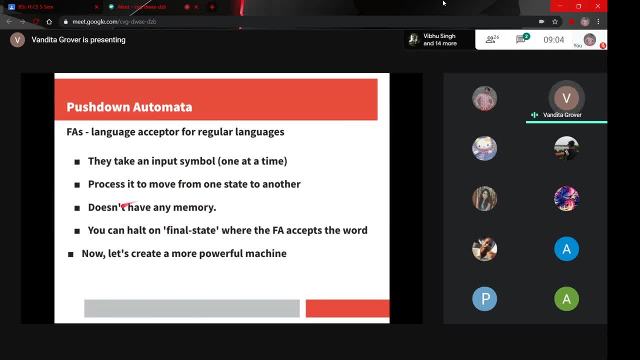 we don't have a memory. we have not talked about any memory. similarly, we are just imagining that the input is coming in the in a stream, so there is some place where input is coming, but we are not storing it anywhere. so there is no memory in xa and you can hold on final state jaha. 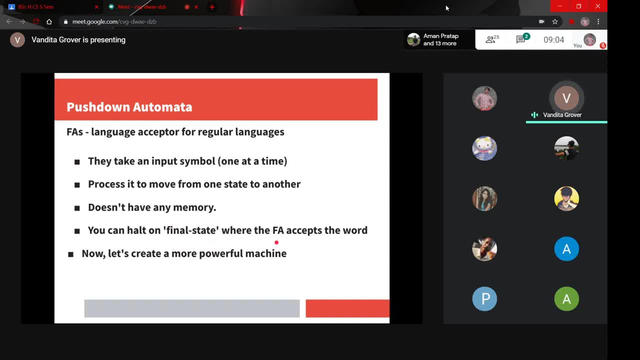 will accept the word. so now we let's try to create a more powerful machine. now let me first introduce the notion of input tape. we which we which we didn't talk about in fa, but this input tape can be applicable in fa also. kahi na kahin to input aega, hi aega. 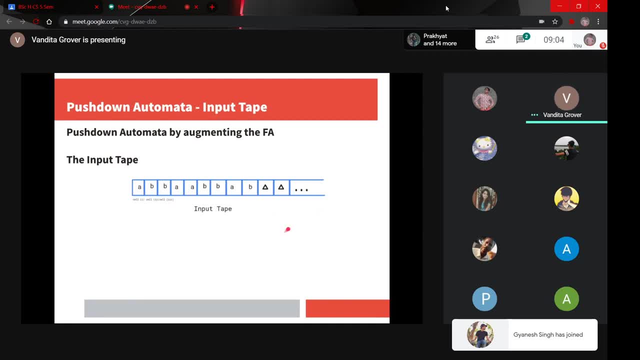 so let's imagine you know a, a tape which is running in an infinite. uh, it is an infinite tape. you will be able to put it on the input, so it contains cells. these things are called cells and initially they are blanks. every for every cell, empty cell- there is a blank symbol. 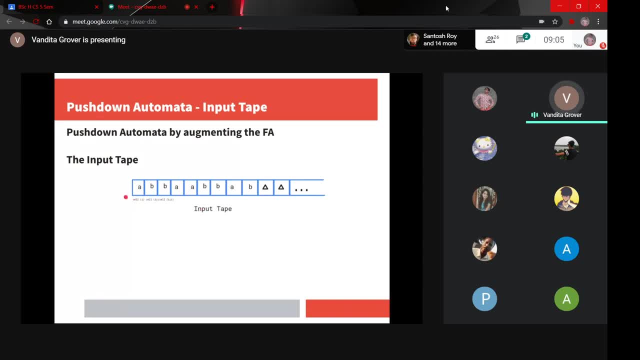 let me call this as a blank symbol. so as soon as the user and put enters the input or whatever input you are going to talk about, you will place one by one on each cell and basically you will be writing the black over, writing the blank symbols to. 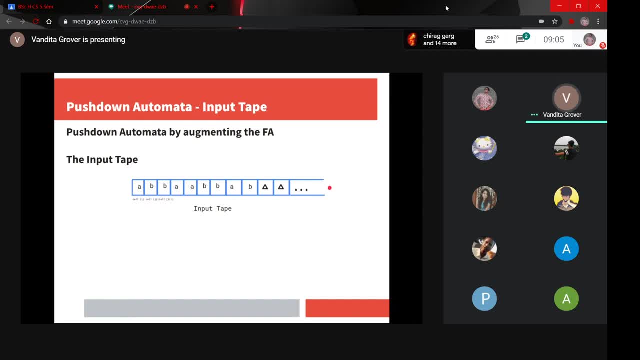 write this and the rest things remains up, remains black. so this is the input tape. so input tape is infinite in one direction and it consists of cells. it consists, contains a star apple, apne input kajal. alphabet: leota was sigma leota. yeah, happy, just tackle for better with. 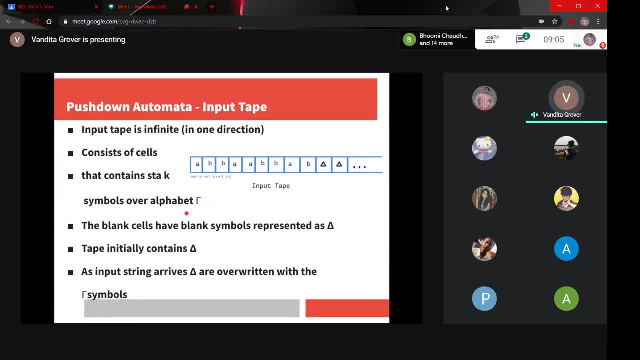 common gamma category. okay, bar to gamma or sigma with a hammer equal. okay, this is a good. a comma, be pay up main define kia to stack you per be a sorry, stack you per be up. Johan. a comma, B comma, whatever you can write that. apart from that, there is one thing extra, which is your blank symbol. yeah, okay, Sigma. 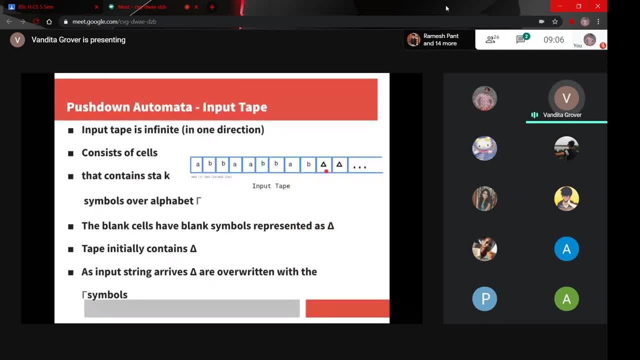 disque para define. you're a language was main blank symbol. like you to make input tape. minimo that so is. he is scales about Conama, gamma rock again. so initially the tape contains blank and as soon as the input comes it gets it. the blunts get over. 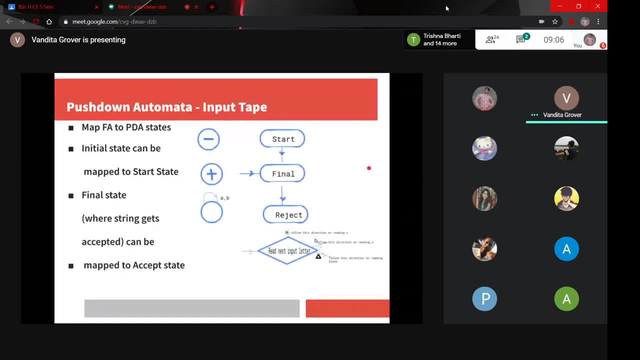 written and the remaining will stay as black. so if I map, you know F is dates to PDS states. so you have initial state which can be mapped to start state. you have a final state which can be mapped to a. a final state to look forever is rejected. 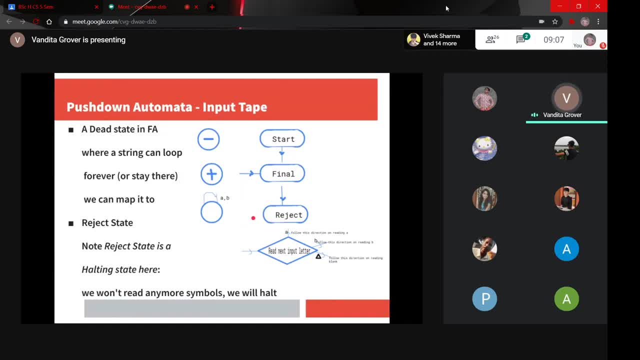 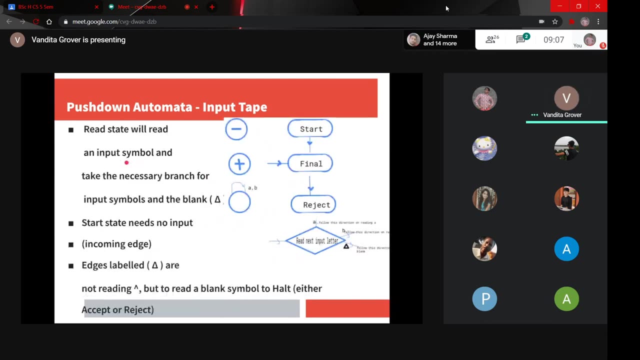 so we are mapping it to accept state, then final state and reject state are halting states. this is for accepting and halting and this is for rejecting and halting, so we call them halting states. after that you have read state. so all input symbols like A and B. 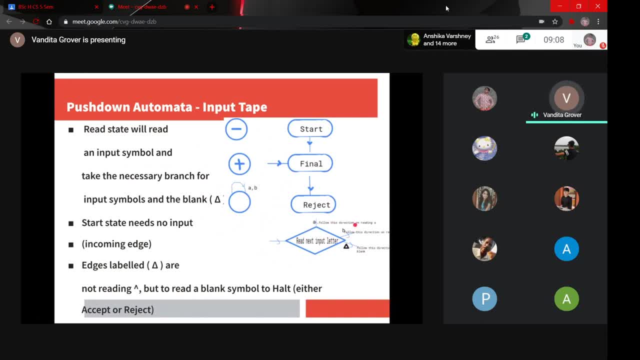 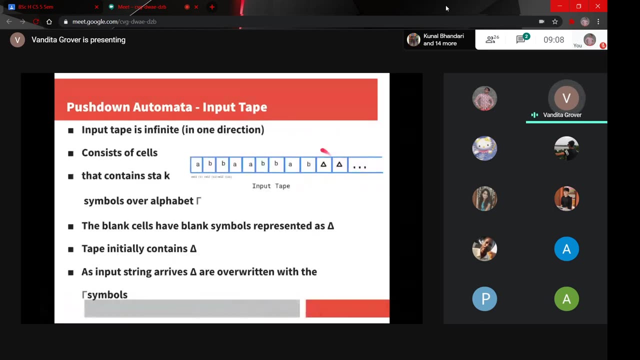 will have same direction. if A comes, then do this, if B comes, then do this, so all the input symbols will have same possible direction. apart from that, blank encounter happens on input tape because your input tape was this, so when it will read and sometimes blank encounter happens. 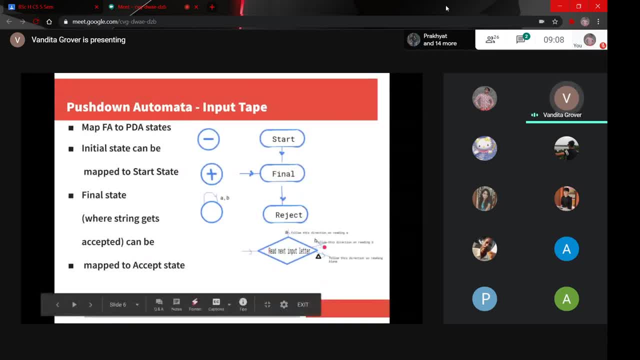 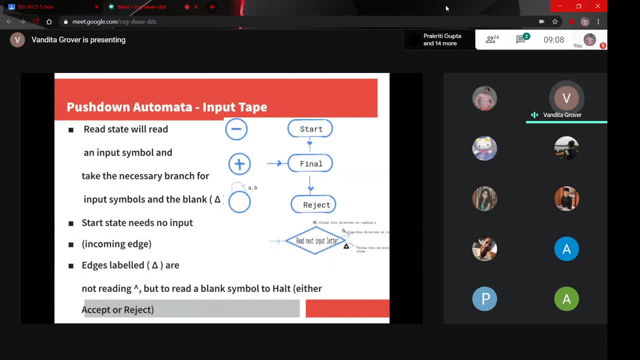 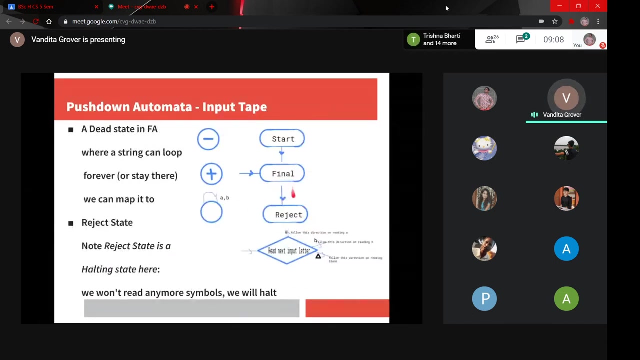 so it will have same direction. so read the next letter and blank direction. so this is how the states will look like. so in PDA and FA, everything is same. there is also input tape. sorry, there is also input tape. you have mapped all the states at start and final. 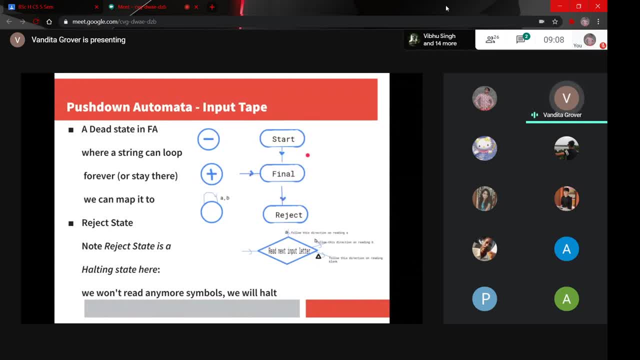 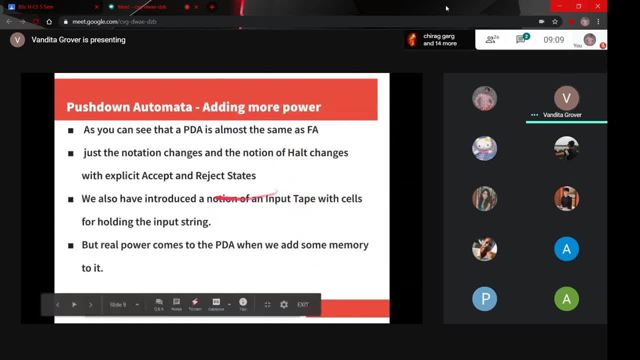 and you have introduced two notions of halting state. either it will be accepted and halting, or it will be rejected and halting. then you have made a different state for reading. so it is almost same to FA means whatever was accepted in FA can be accepted in FA. 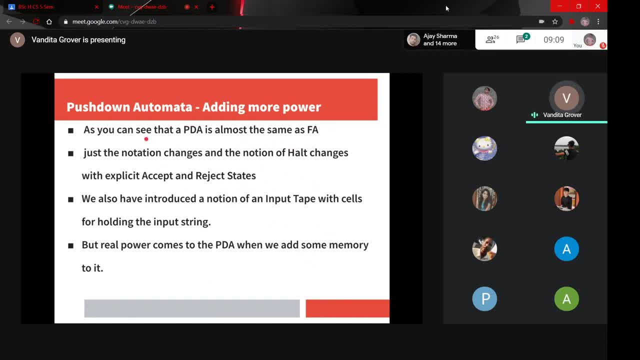 means FA of regular language can be accepted, so PDA of regular language can also be accepted. but if it is same, then what have we done? so now, what we will do? we will give memory to this PDA, which was not there in FA. I am adding more power to it. 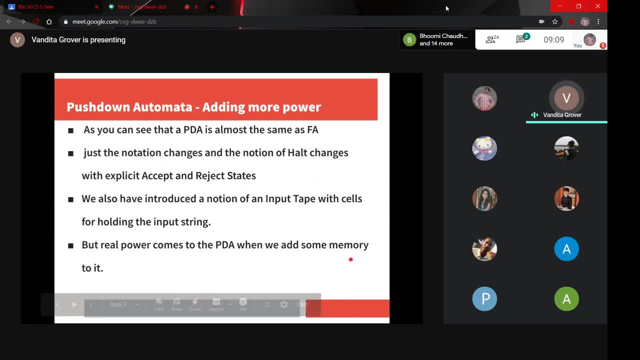 by giving memory. now many students say that they have given input tape, but that is not the power, because we assume that there is an input tape in FA. we did not talk about that, so input tape is not giving you more power. this memory is giving you more power. 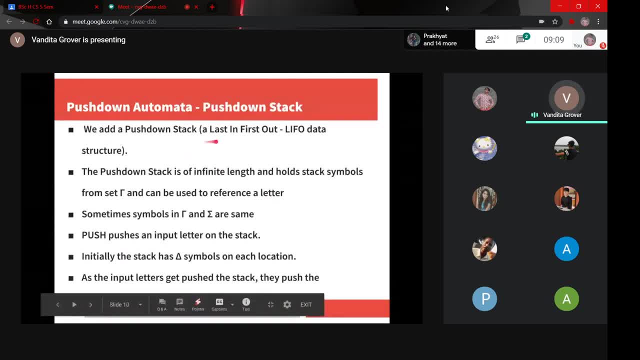 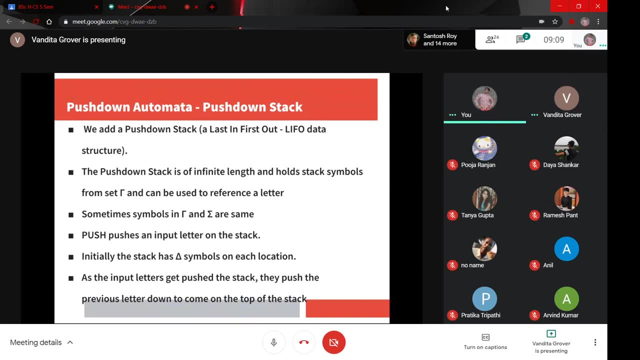 so we have given a stack to give that memory. what is a stack? does anyone remember what is a stack? look at it and tell me. ok, what do you do in a stack? are you studying data structure, I guess. so what is what is stack doing? what are? 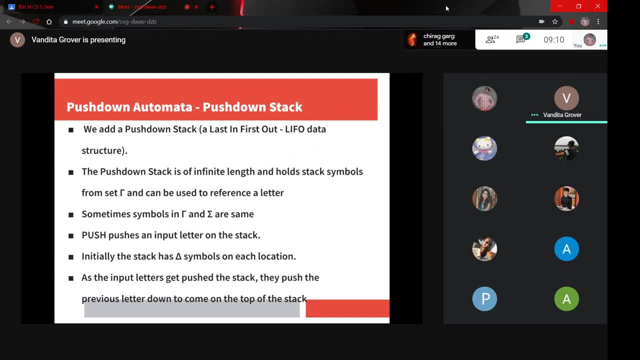 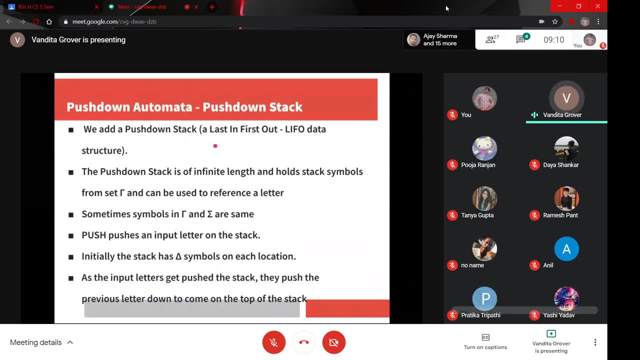 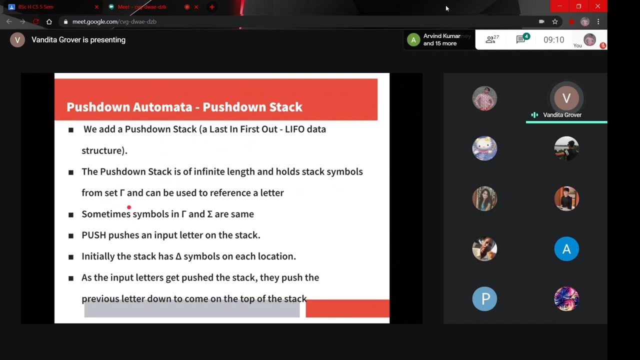 so what are the operations of stack? ok, so we have a special memory data structure which is called push down stack, last in, first out. push down stack is of infinite length and stack symbols, because stack set we made gamma. so sometimes what happens is we are giving a comma b on input tape. 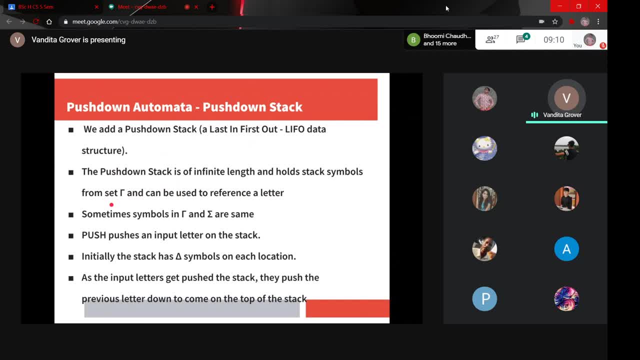 but in stack we are writing 0 and 1. that works. so sigma would be a comma b and gamma would be 0 comma 1. this is possible, but in gamma a comma b can be, so we can say that sigma is equal to a comma b. 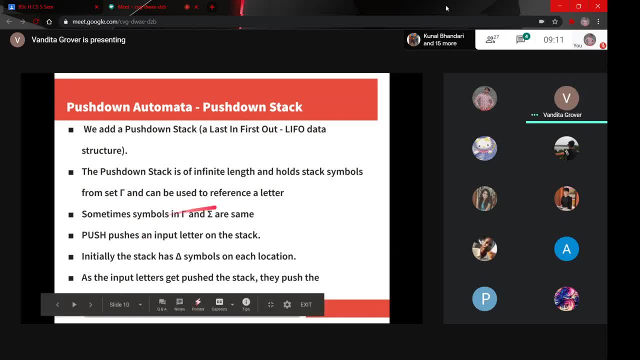 and gamma is also a comma b, added to that a blank symbol. so gamma is used to reference a letter on the input tape and put it inside the stack. sometimes the symbols are same. push will push an input letter on the stack. initially, in stack also there are blank symbols. 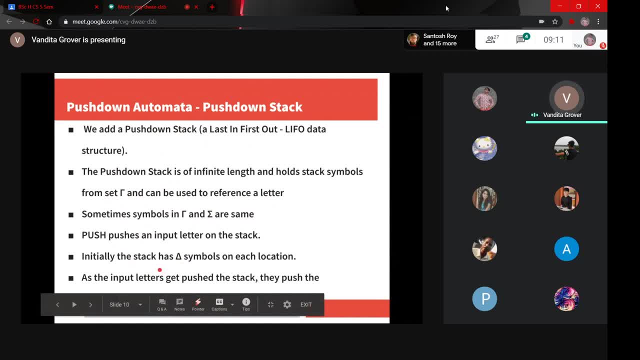 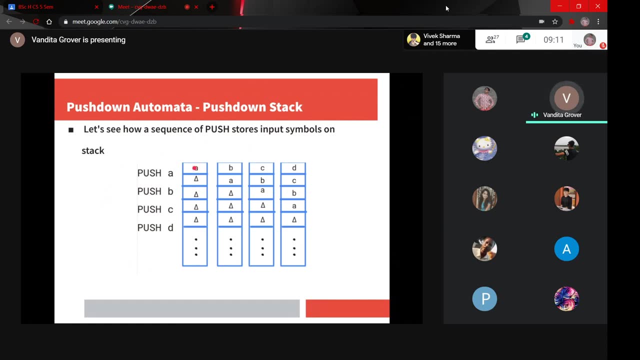 and as you keep pushing the input letters, it keeps pushing down and the last element is always on top. you know the basic definition of stack. so if I push a, the entire stack was blank. if I push a, the stack looks like this: if I push b, the stack looks like this: 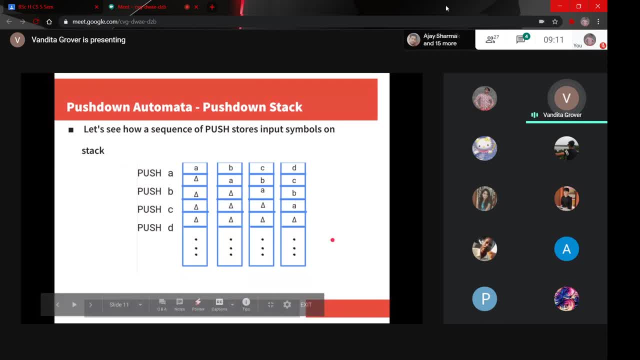 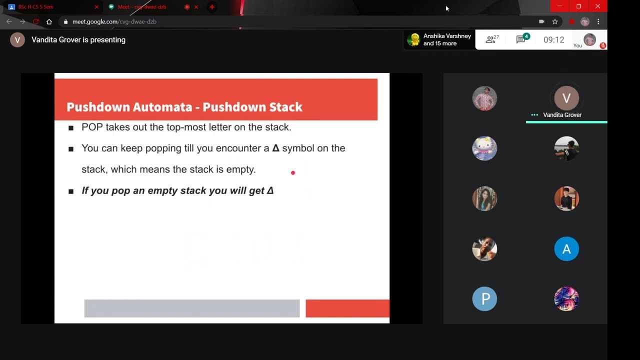 if I push c, the stack looks like this: if I push d, the stack looks like this. I think this is very clear. in pop you will get the topmost letter. so if you will pop, see there is a choice while pushing a or b, but there is no choice while popping. 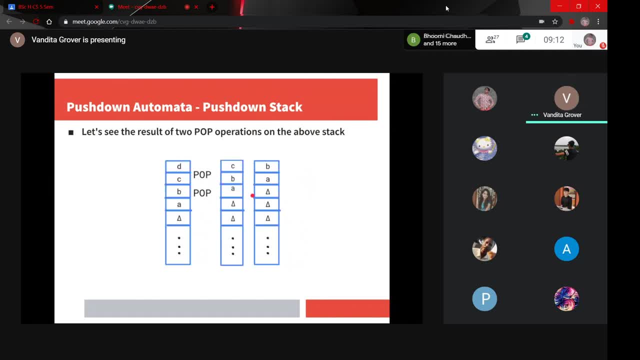 if you pop an empty stack, you will get a blank. so something like this: when you pop first, the stack looks like this. when you pop second, the stack looks like this. is it clear? I hope this is clear if you want to show it in, push down automata. 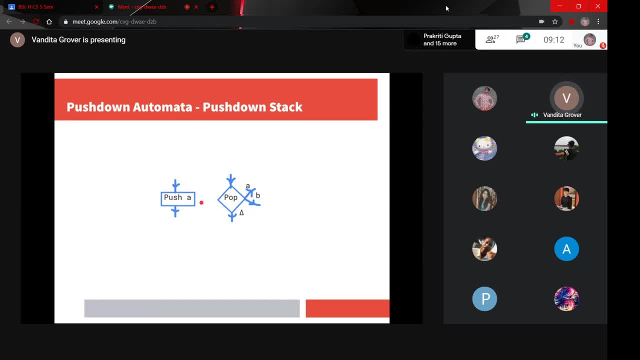 you can make two states: push a and pop. now see here it is very clear that you can push the input. if you want to push b, there has to be a separate state called push b. but while popping we don't know what will pop, so we have to consider all alternatives. 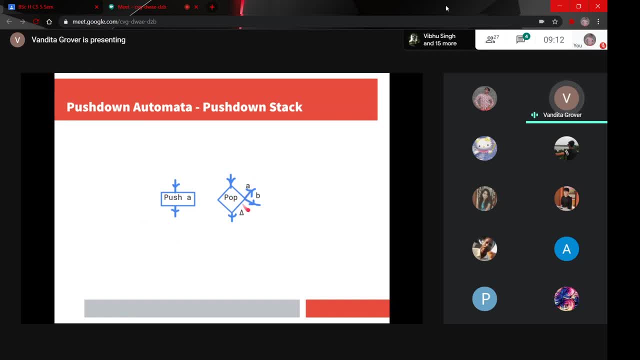 in this case it is one direction because we know what we are pushing, but while popping we don't know. there can be n number of possibilities as the number of letters in the alphabet. so we are giving options in which direction to go, like in flow chart. so we know the input. 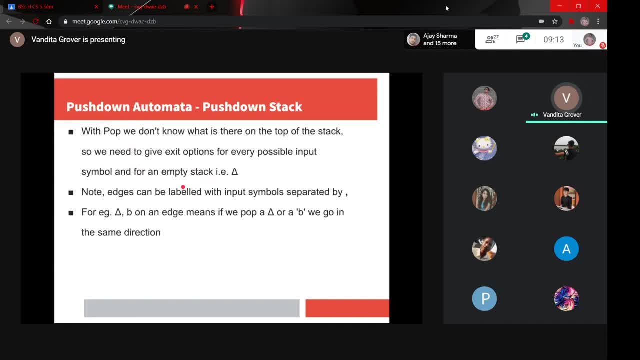 simply want to push. so there is only one entry and one exit with pop. we don't know what is there on the top of the stack, so we have to give all the exit options. so this is an essay. you have read this essay. given the information I have given you now. 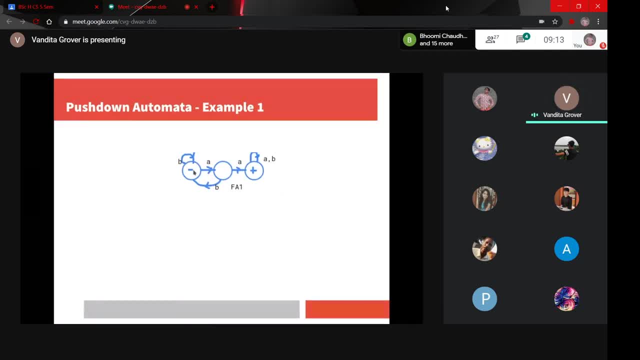 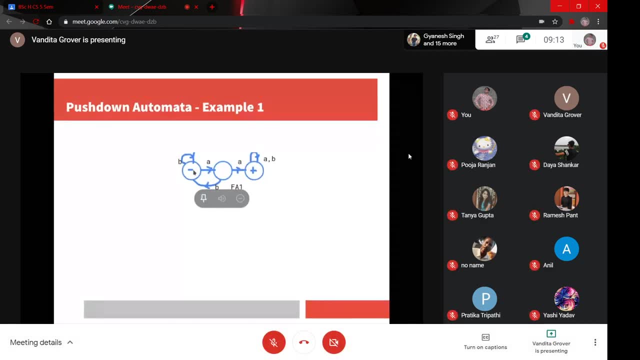 I want you to draw a finite automata for this. please, please, please, please, draw a finite automata for this diagram. I am giving you 5 minutes time. please draw it on pen and paper, using other states that I have already told you and using the stack. 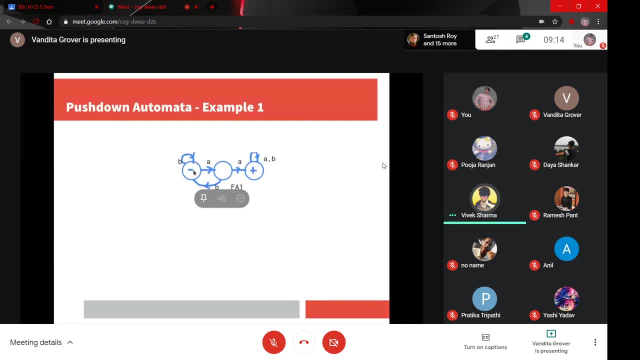 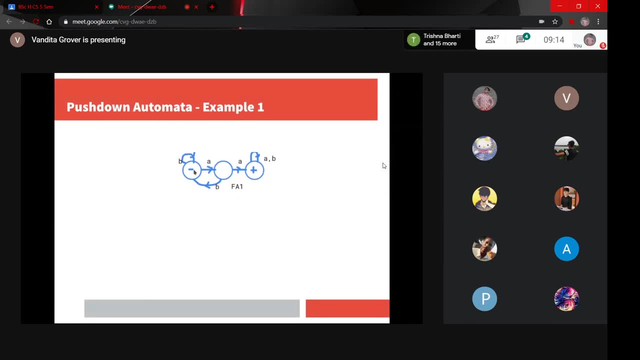 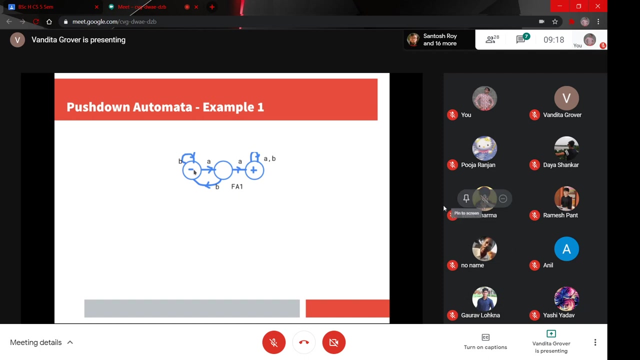 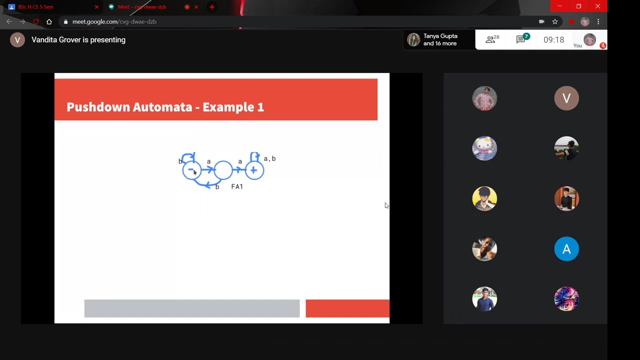 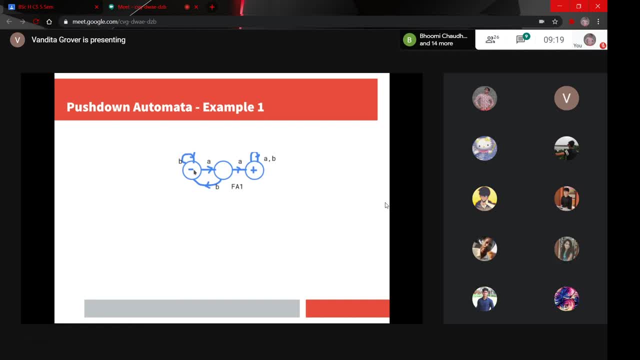 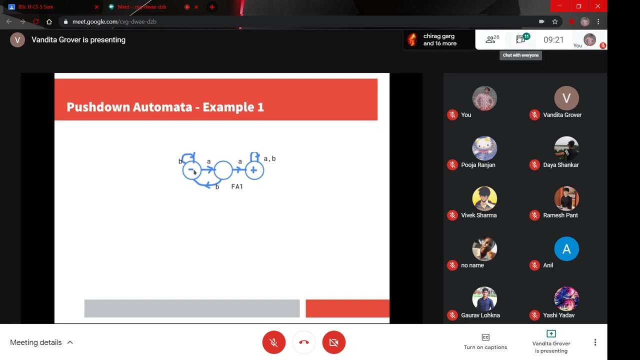 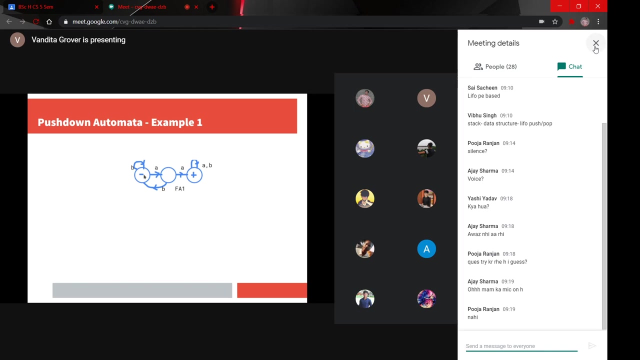 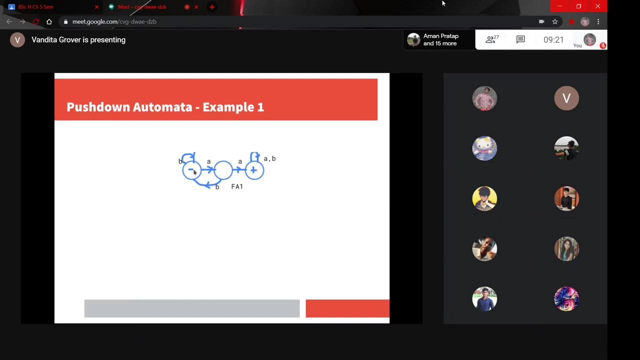 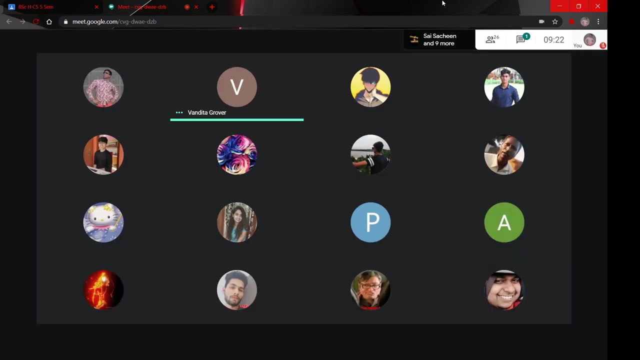 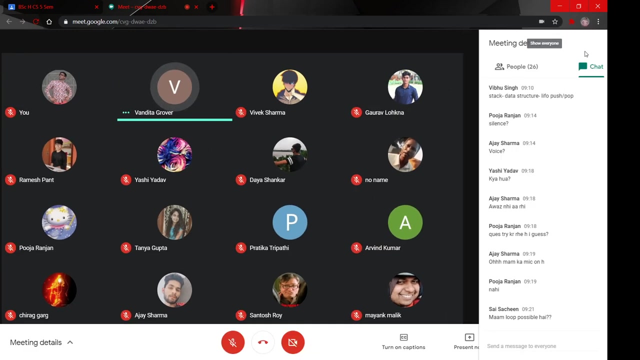 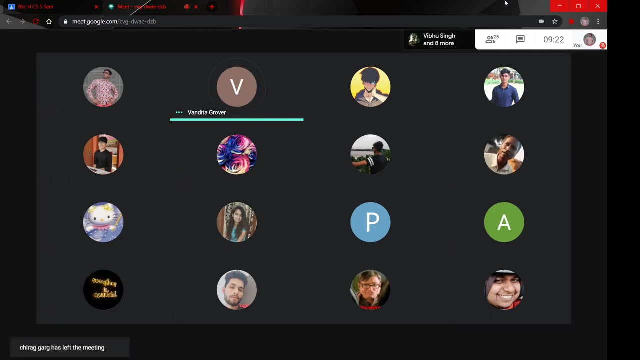 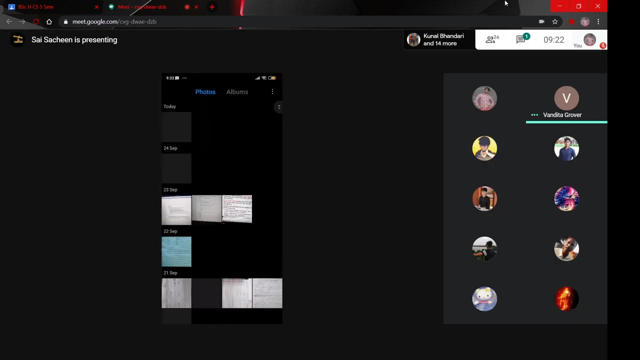 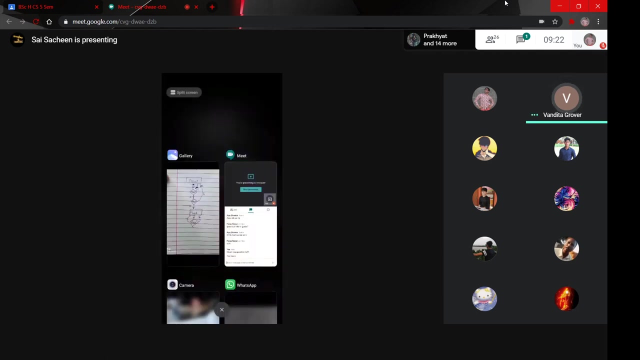 you, you, you, you, you, okay done please. yeah, loop is possible, sachin, are you done? please show what you have done. so i stopped presenting one of you. show me the screens that you have done. okay, can you unmute yourself? you have done start. yes, ma'am. 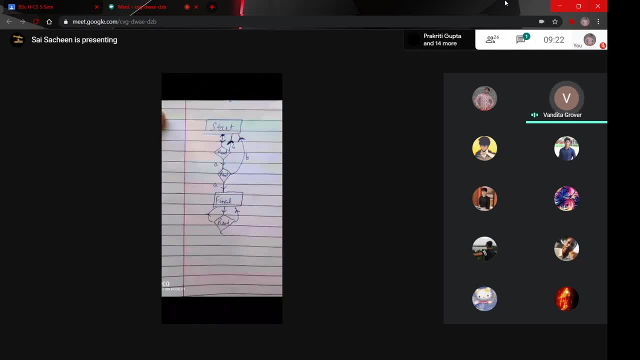 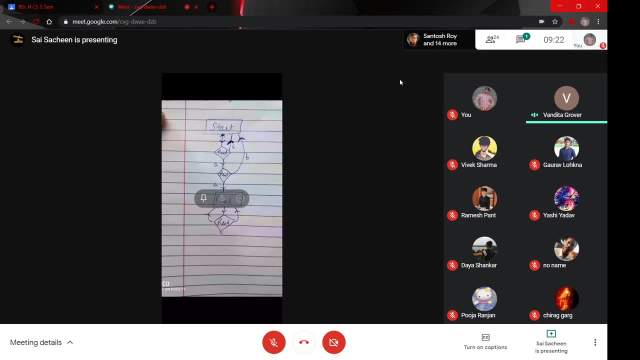 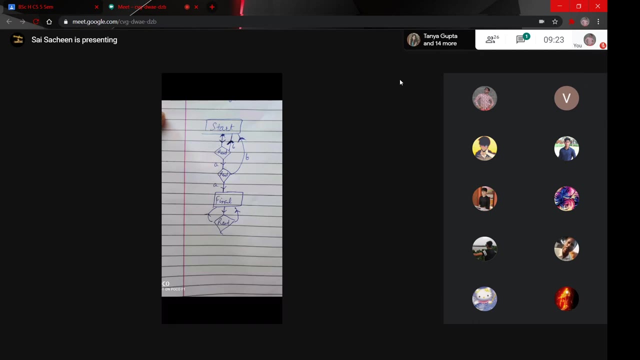 you've done a start, then you have read an a and then, if you read an a, okay. so when you're reading a b, why are you going back to the start, ma'am? because, uh, on the it has, it has given a loop for starting, so we are not moving to next state. so, instead of you know, 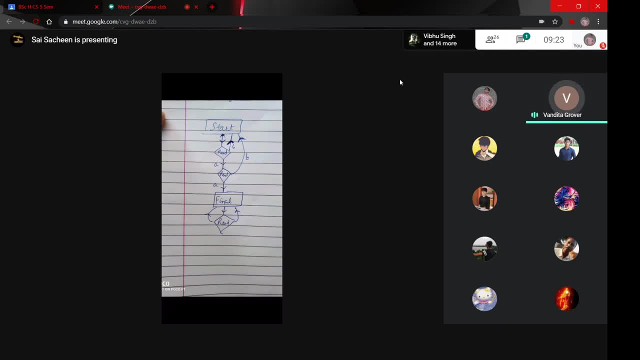 moving from start because it is a loop. just put this arrow. uh, don't go on the start state, don't go back to the start set. connect this arrow with the arrow just above the read. so start for touching arrows. okay, then you have a, a, b next. 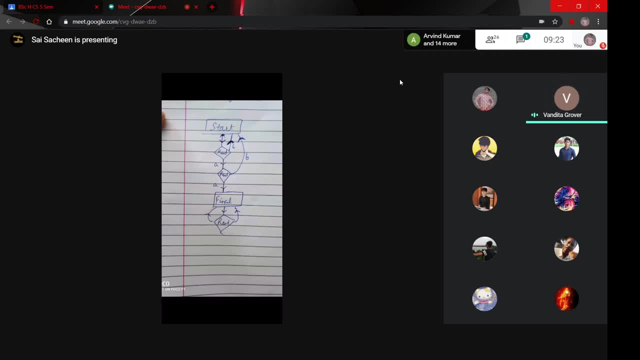 it has a loop for this moment, and now we search theboots and i did this. you are looking good, but when you actually touch the boots, then that you won't look back. you go to the durchaus as if you have done it. you can even 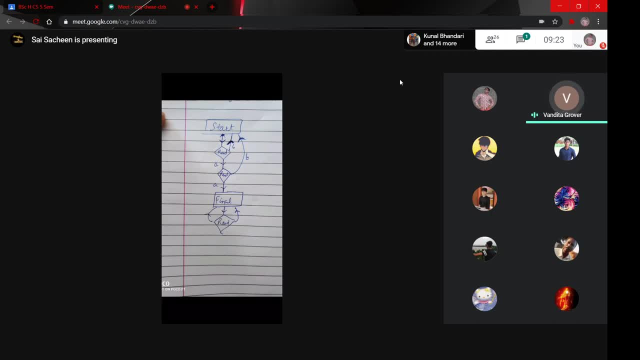 so when they will plan, because they don't know the story, i'm going to them, so if you likewise, you can call them okay. yes, she said not. okay. well, it's okay, do it, because in a couple of days it does not work like you always do for the rest of your life. 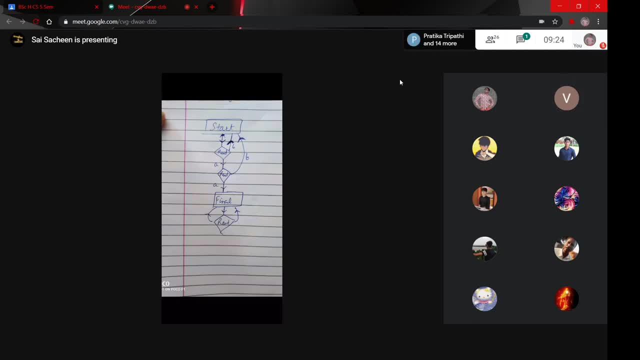 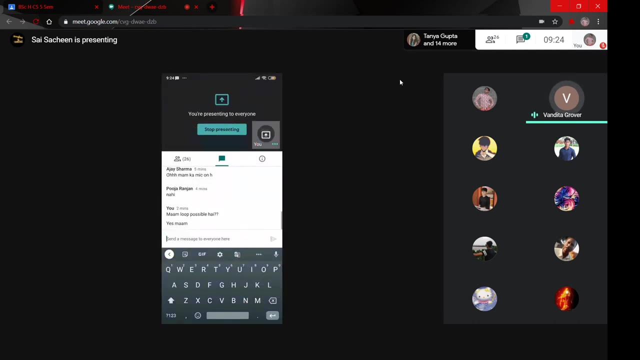 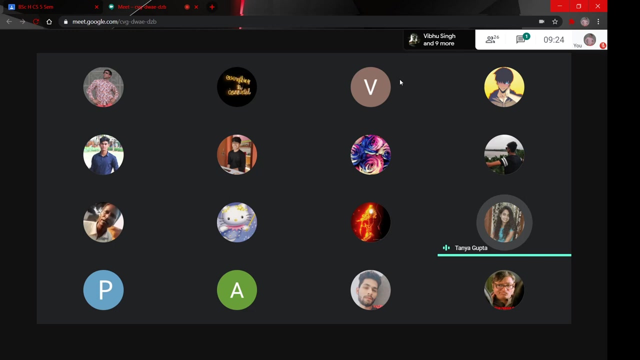 Just think about it. what if a lot of A's and B's? how will you make A plus B's target acceptable? Just think about it. Anyone else who wants to present? Okay, ma'am, Thank you. Thank you, Done. 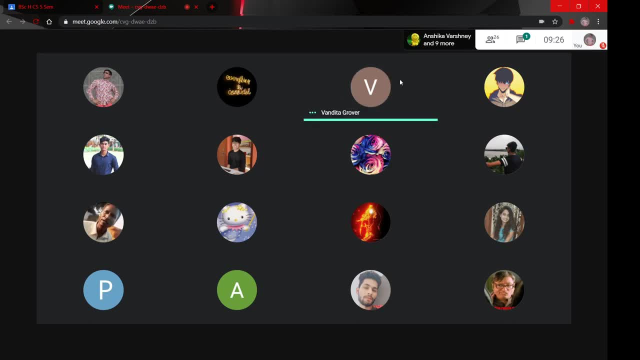 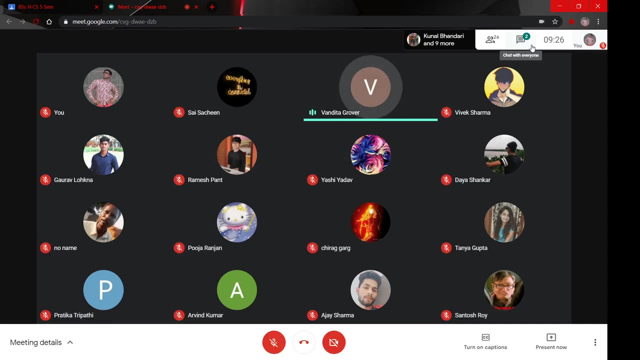 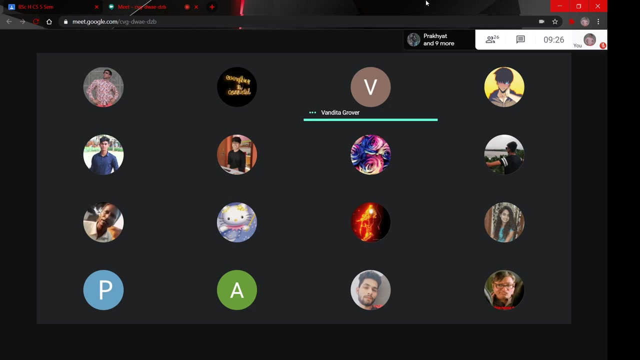 Anyone tried Okay, Thank you. Did anyone try Okay? Did anyone try Okay? Did anyone try Okay? I don't know how many people will make A plus B's target. I don't know if I can do it. 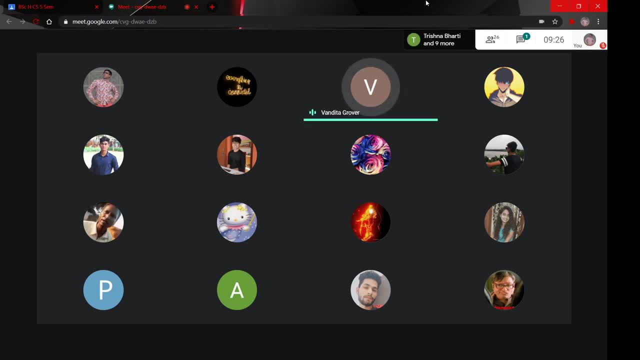 Thank you. Okay, ma'am, I will try. SPEAKER 2 SPEAKER 3 SPEAKER 3 SPEAKER 4 SPEAKER 3 SPEAKER 5 SPEAKER 6 SPEAKER 10 SPEAKER 11 SPEAKER 12. 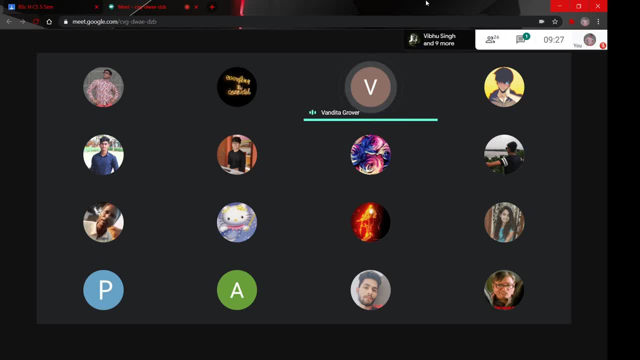 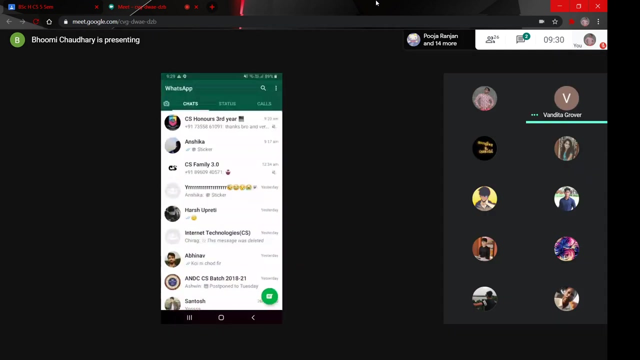 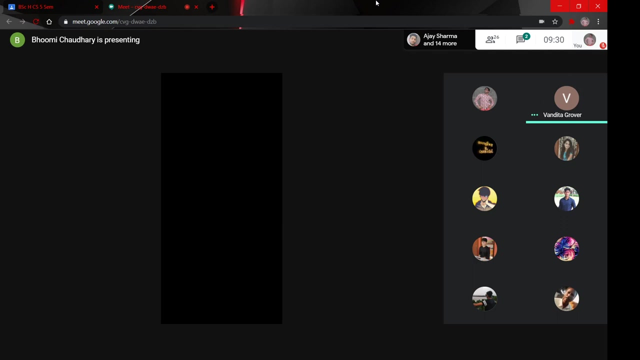 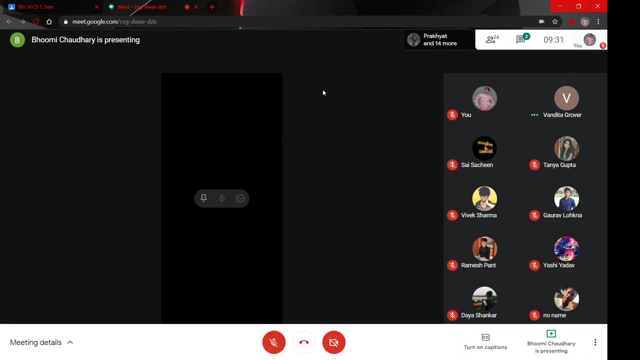 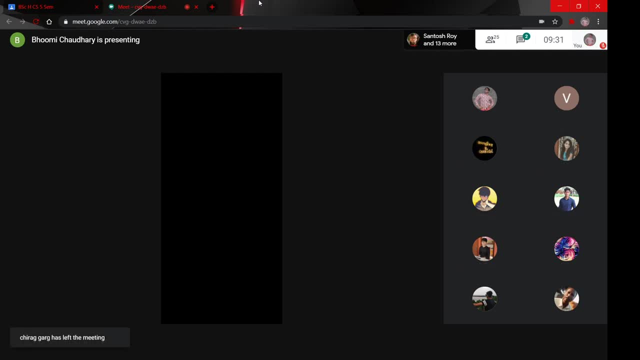 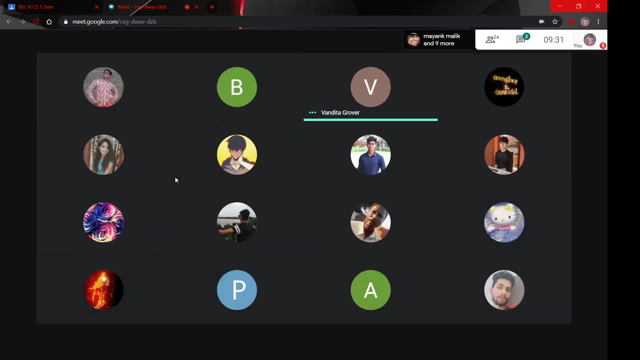 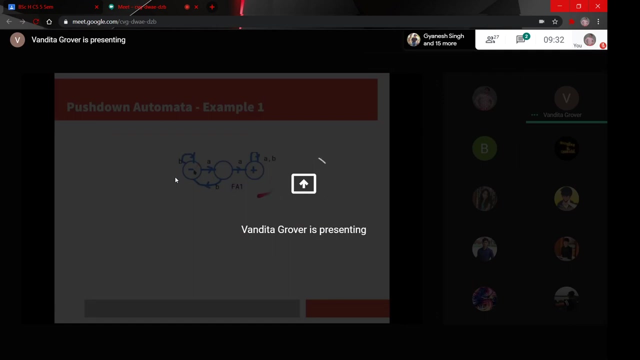 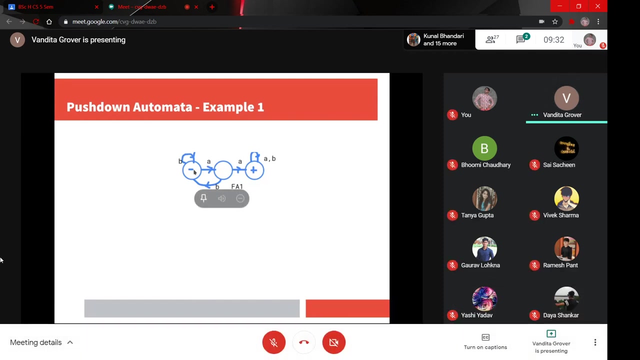 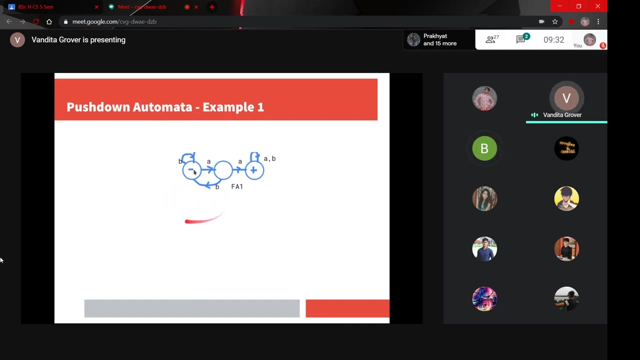 Thank you. Thank you. We are pushing B in the initial state as well. This is a loop. It simply means that if B comes, I stay in this state. It is being pushed in the intermediate state as well. Tell me one thing: is F in stack? 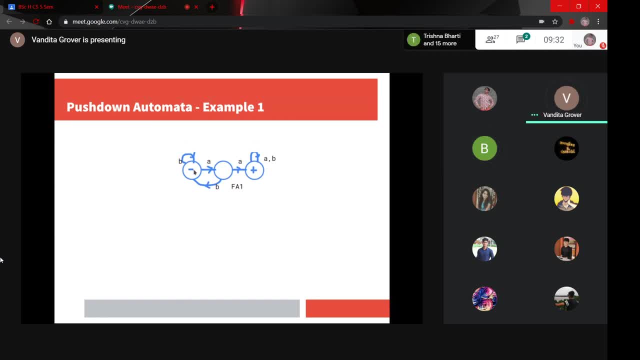 Yes, Are you sure? I am confused. What is the difference between B and F in Bhoomi? What is the difference between push down automata and F in Bhoomi? You told me that memory is used in Bhoomi and push down automata is used in Bhoomi. 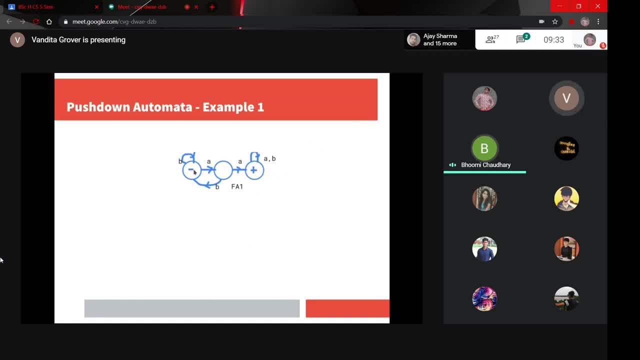 Is F in Bhoomi used in Bhoomi? No, Then it is not possible to push down automata in Bhoomi, right? No? So what are you doing now? No, If input A is coming, then you are transitioning between states. 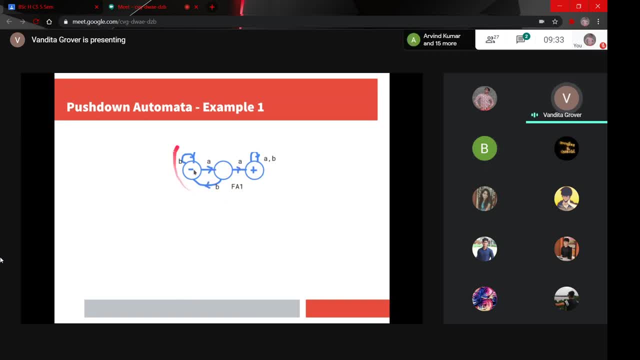 You are going from one state to another state, or you are going from one state to another state, or you are staying in this state, or you are going out of this state, or whatever. So this is what you are doing, Okay. What do you say? 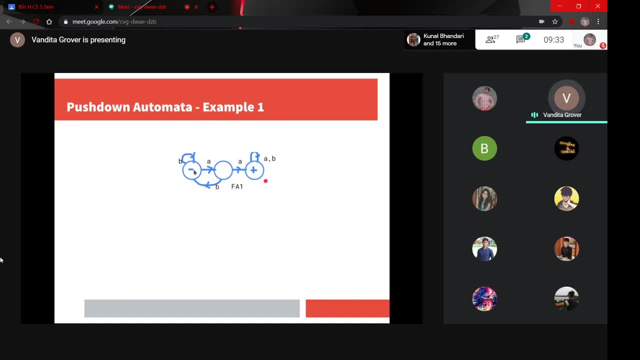 Push down automata. But we told you to make the same thing with PDA- Push down automata. So when you made the same thing with push down automata, then you- which Sachin just said- you made something like this: 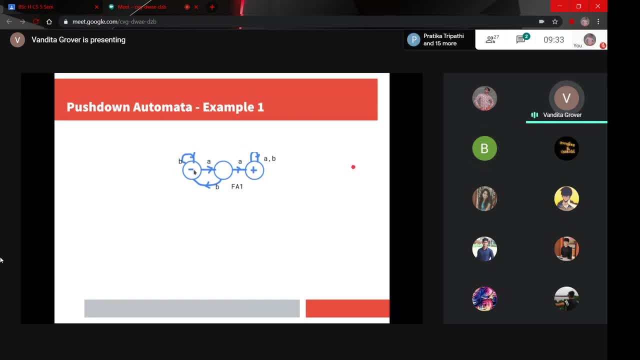 When there is no need for stack in this, then do you need to use stack in push down automata. When there is no need for stack in this, then do you need to use stack in push down automata. You don't need a stack to express this language. 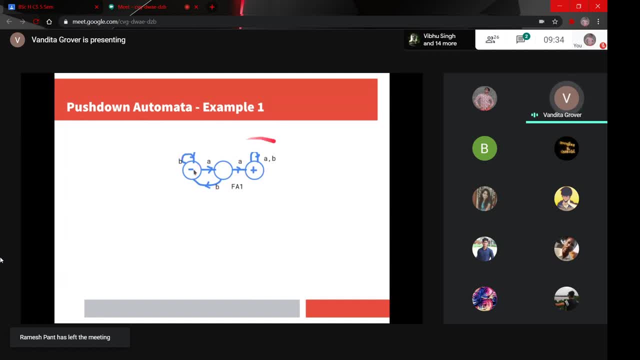 Because that's why you could create an FA. It was regular, So you could make an FA And you don't need a stack. Having said that, push down automata has a stack, But it is necessary. It is not necessary that if there are 3 rooms in your house and you use 2 rooms, then it is not necessary that you use that room. 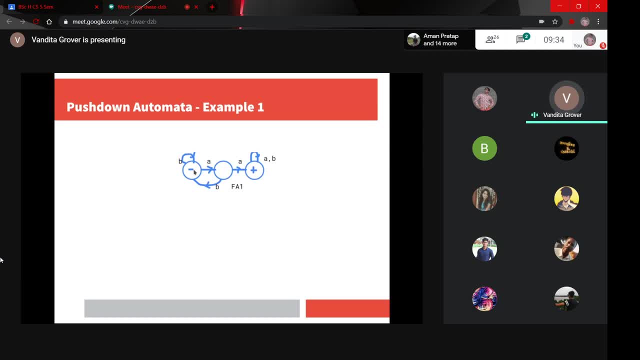 You have extra power Just in case something new comes, then most likely you will keep it in your third room. But if you don't need it, you will not keep it in the third room, right? So it is something of the same sort. 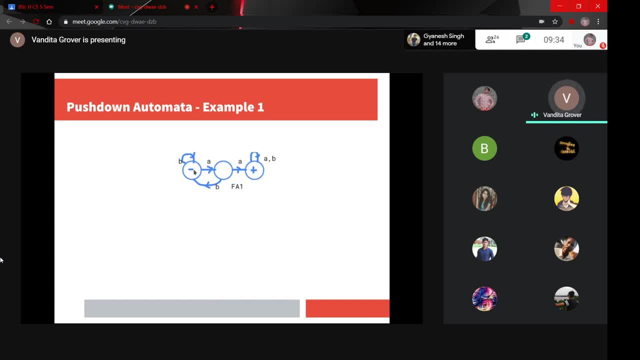 Yes, we have a power in push-down automata, power of an extra memory space known as the stack, but I don't need it So I will not use it as you have done. So this is the final push-down automata. 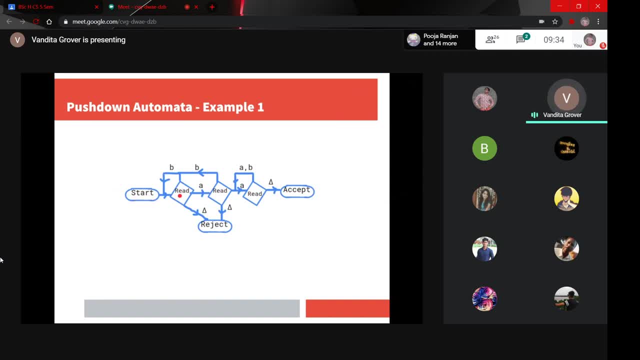 You go in the start state. You read: If you read an A, you read the next state. If you read an A, you move to the next state. But if you read a B, you keep on looping in this state, In the next state. if you read a B, you keep on looping here. 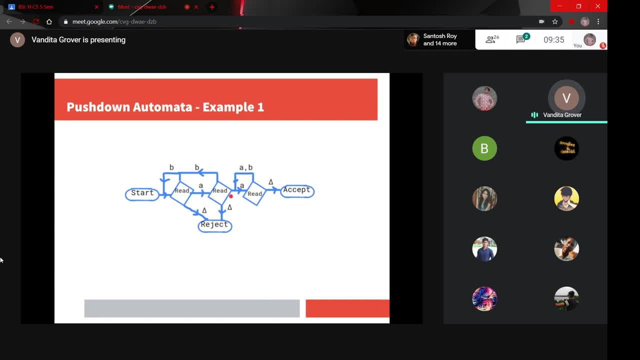 After that, because you need double A like this: if double A comes, then you go to the last read state. If you go to the last read state, then whatever A and B come, because I only needed double A, whatever A and B come, I will keep on looping here. 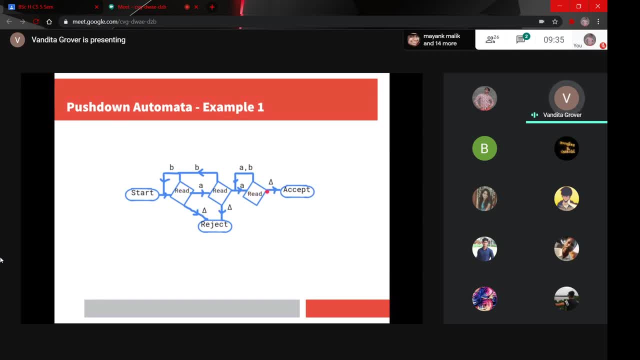 And as soon as the symbols on the input tape are finished, that is, if you get blank, then I will accept it, because I got my double A. Apart from that, anything is coming. for example, blank is coming, or anything is coming. 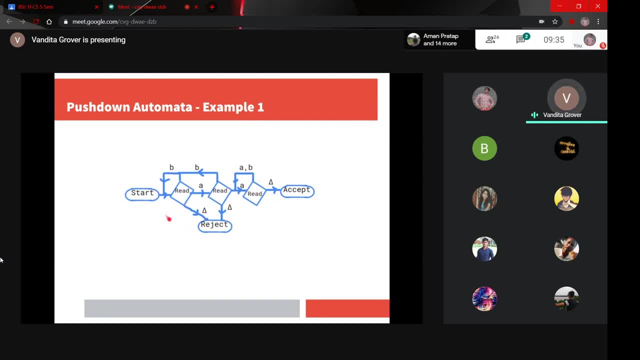 because you need double A in the language. So if the input symbol is blank or simple B or only A, in that case you will go to the reject state. Is this clear, Ma'am? the last read of A and B that you made. 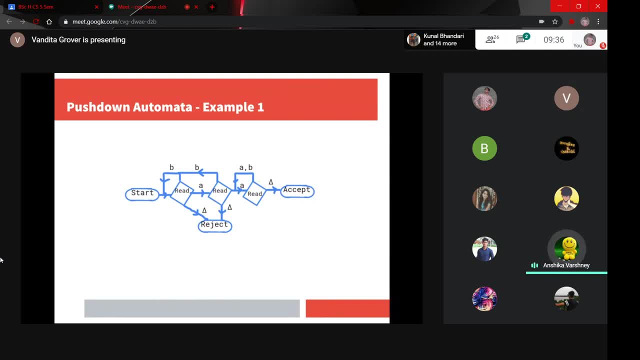 like in FA, that loop is in the final state. So why did you make it on read? Because in FA you can make it in the final state. What happens in FA in this? When you go to the final state, then you can also move out of the final state. 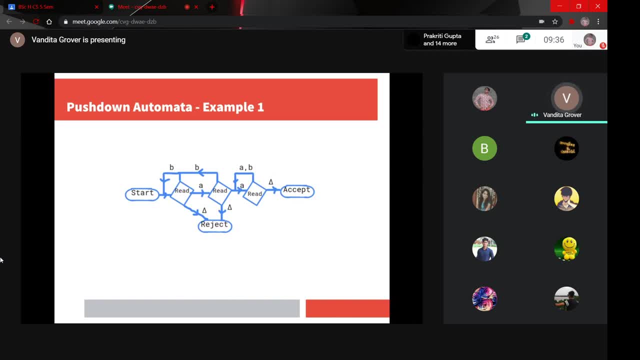 Here and there you can go back to some back state, But in pushdown automata the main difference is that your clear accept state is there. The accept and reject state is the halt state. Once you go into this, you will not go out. 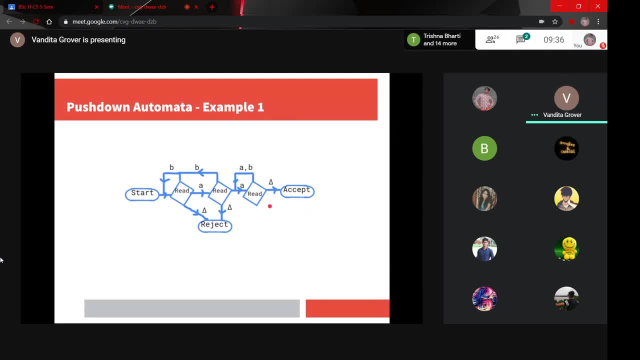 So whatever processing you have to do, do it before that. That is why it was not made in the final state. The job of this and this state is to halt. In this case, accept and reject. In this case, accept the string and halt. 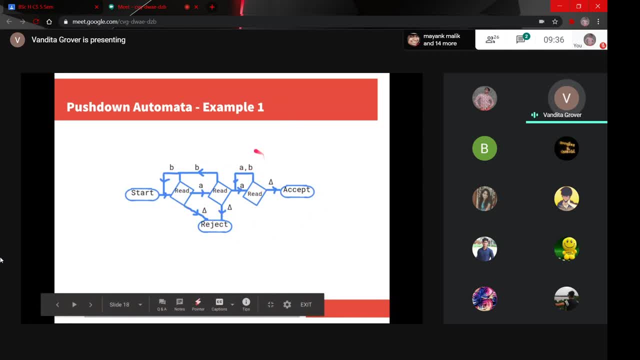 And, in this case, reject the string and halt. So, whatever processing you have to do, do it here, And there was no such requirement in FA. Is this clear? Is this example clear, Ma'am? Yes, ma'am, Ma'am. the last read of A and B. 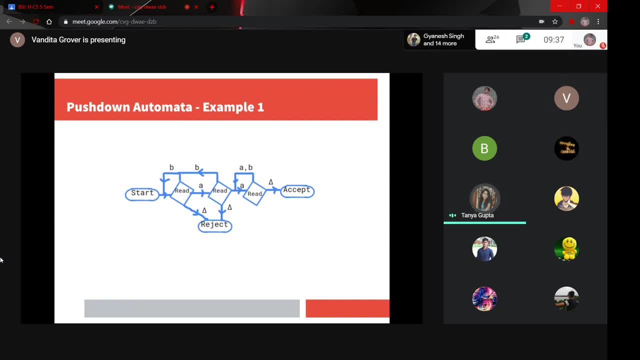 if we accept B here and if we give A in the arrow, we will not have any ambiguity. What did you say again? I mean the look that we showed, the one with A and B. Just a second, I will just go and read it. 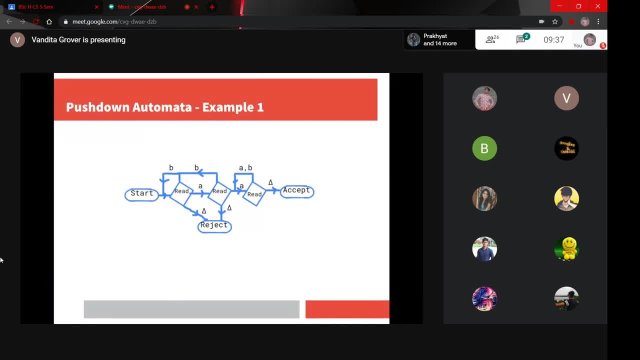 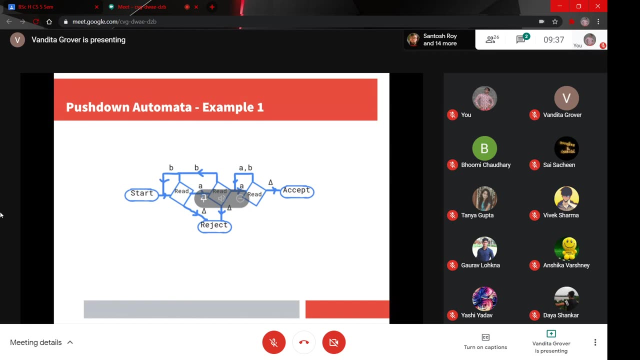 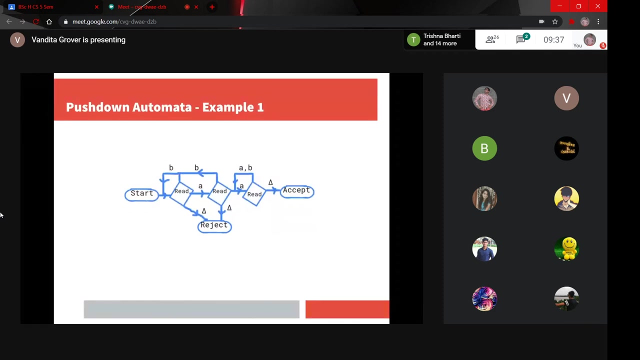 Just a second. Okay, Okay, Okay, Thank you very much. Okay, thank you very much. Thank you for the presentation. You're welcome. Thank you, sir. Thank you so much. You're all welcome. Okay, Thank you for your time. 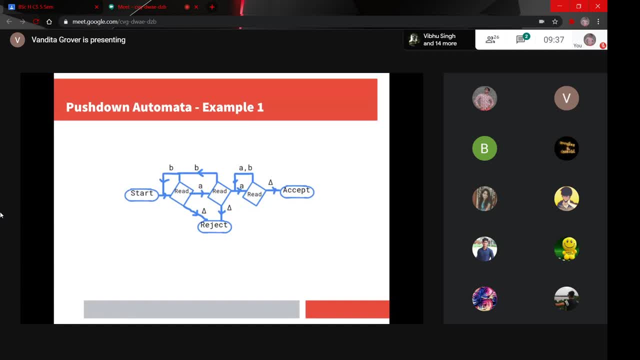 Lester. Thank you, ma'am, You're welcome. Thank you, Thank you, sir. You're welcome. Thank you, sir. Bye-bye everybody. Thank you, Thank you, Thank you So. Thank you, sir. 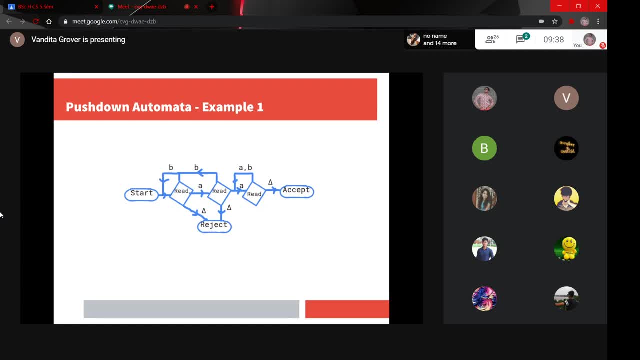 Thank you. It looks like that's the end of our session. The next session is about to end, So we'll end it there and we'll just continue. See you later. everyone you sorry? uh, yeah, so sorry. can you ask me the question again? this is: you are saying this is an a. 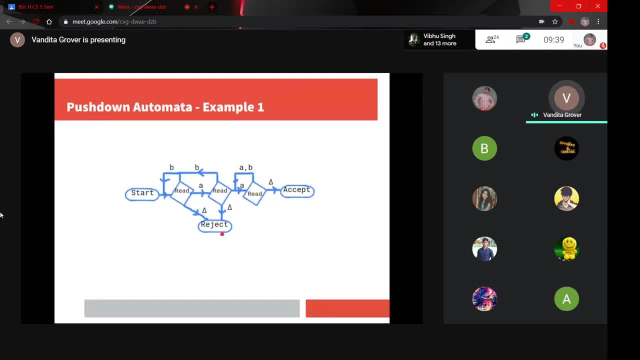 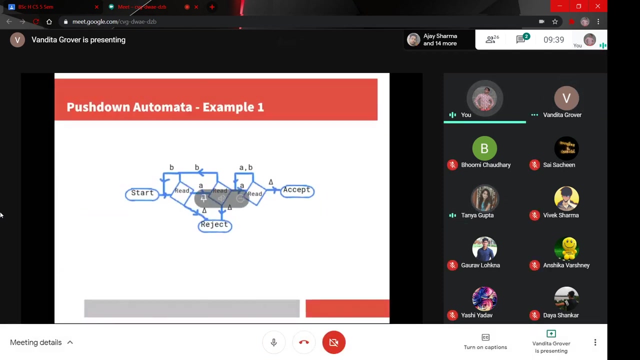 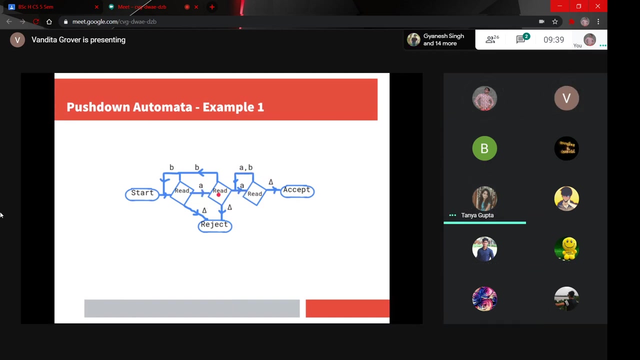 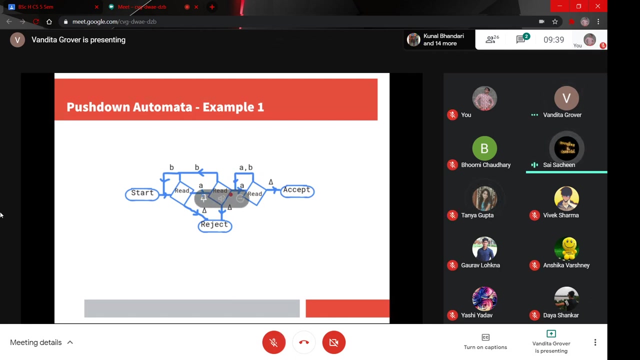 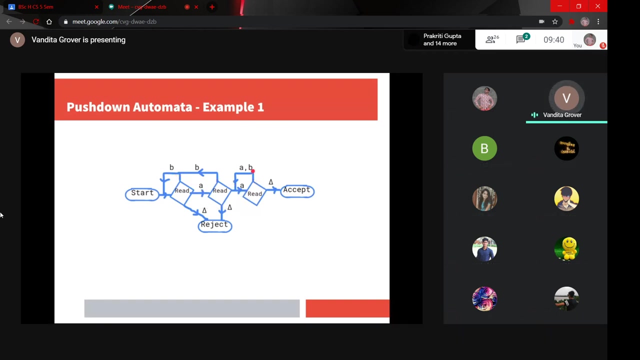 you are building a comma b. so what is the ambiguity? um, um, um, um, um um. Just imagine that this is not here. instead, it is here. you know, arrow is here and A is here. So what is happening is that this edge, this edge's label, this edge is different. 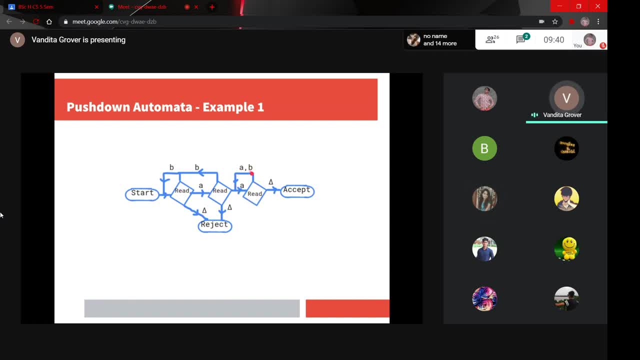 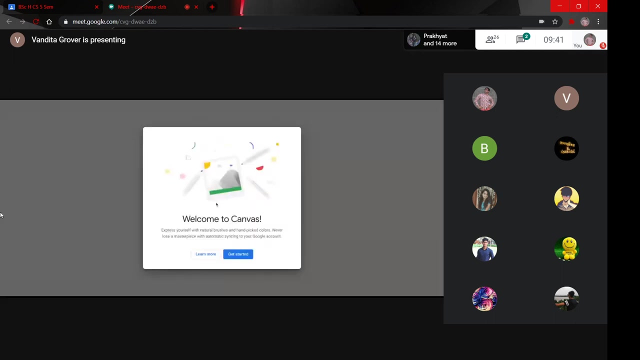 you know, you are saying that this edge is different, this edge is different. you remove this edge. you do something like this. I mean, we are saying that this edge has a point, it draws. Can you see my tab here? 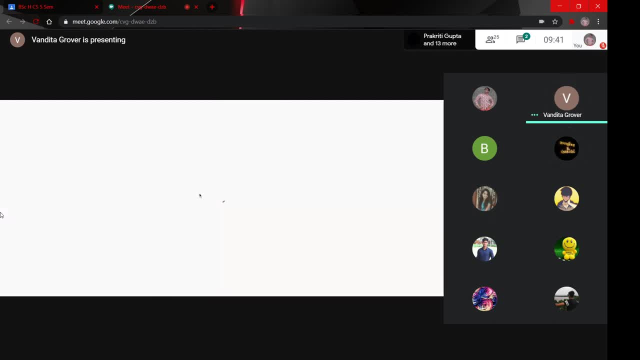 Yes, ma'am, The other one, the canvas tab, can you see? Yes, ma'am, it's loading. So why is it giving me points? and why is it not giving me points, I don't know why. can anyone help me with this? This is not giving me a line and it's just giving me points. I don't know what's happening. 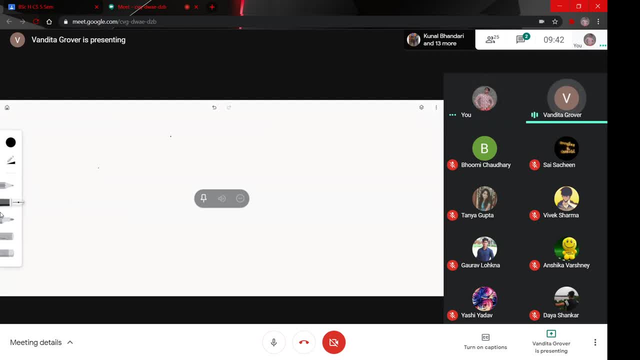 Right, I am using it with the, just that the system is different. I don't have my own system. that's why I am a bit uncomfortable. Sorry for that, but I am probably so. this is for opacity. This line is not being selected, right. 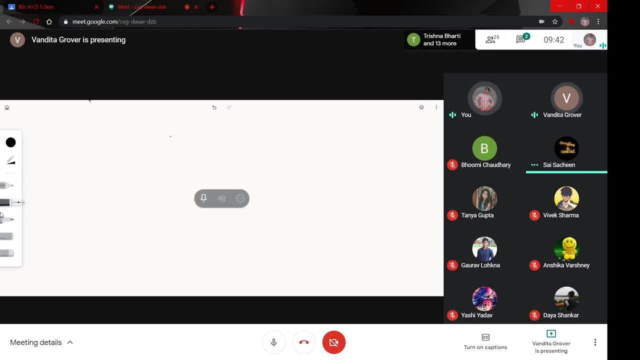 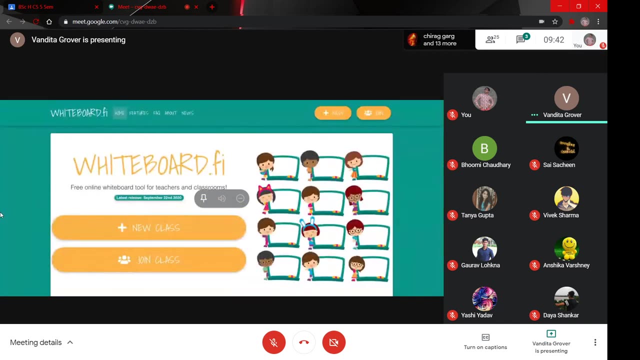 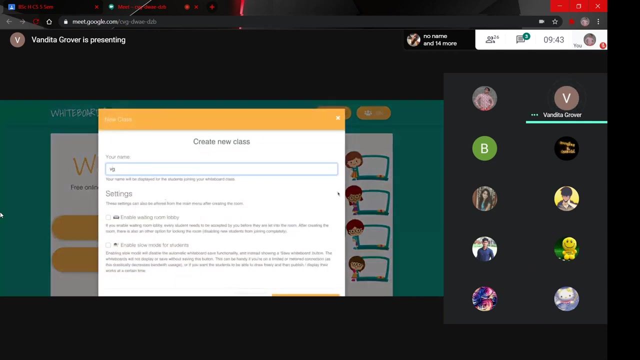 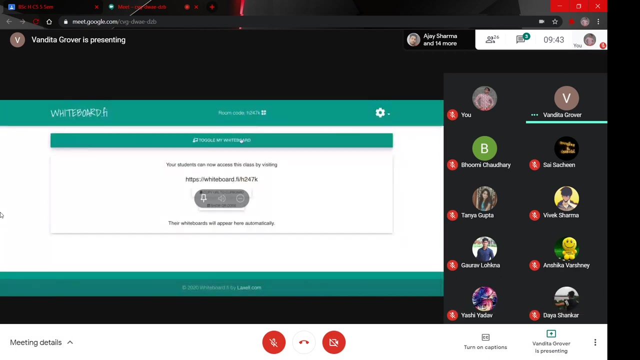 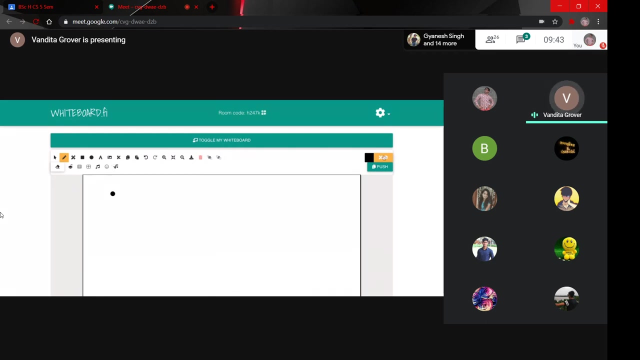 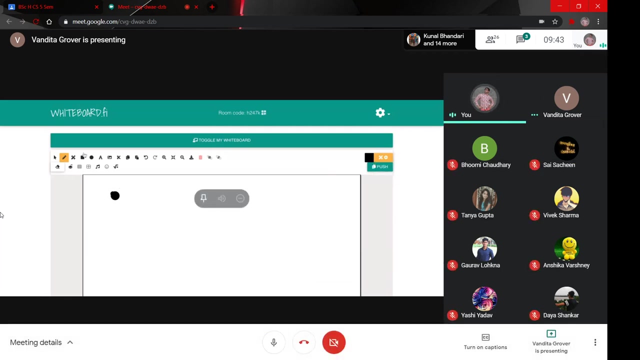 Ma'am, try painting if you have a problem with this. Yaar, this is lagging. Everything is a point. In Mac, things are different. right? My Mac, my system is lagging. I don't understand this. I don't know how to use Mac. I can understand things easily. 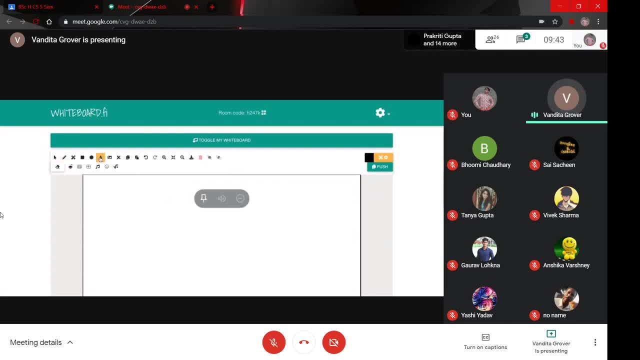 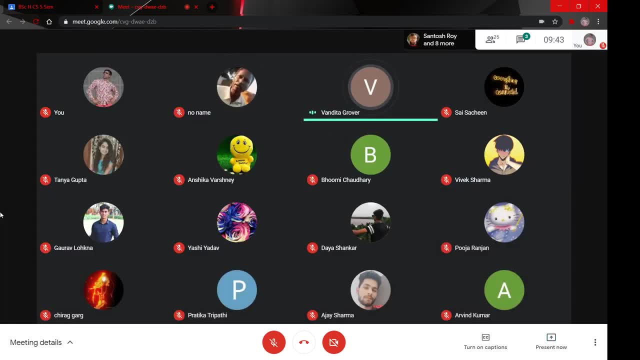 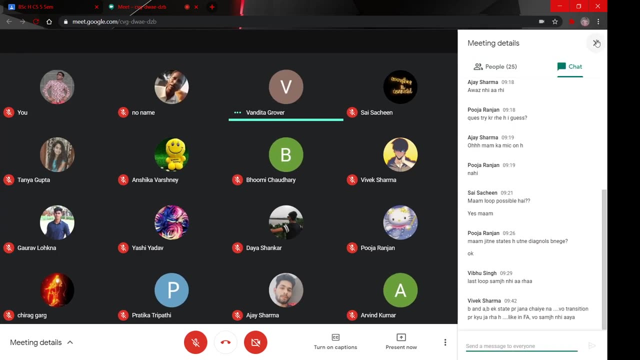 I don't know, I am just. I am so clueless of what is happening. right, We will work on the Mac Windows. I can't work on the Windows Mac, Okay. Okay, there are some pointers here in Google Slides. 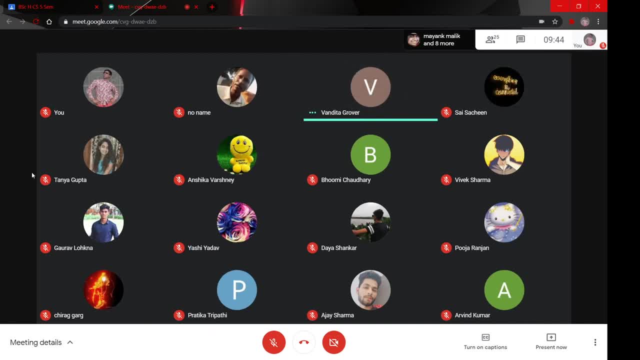 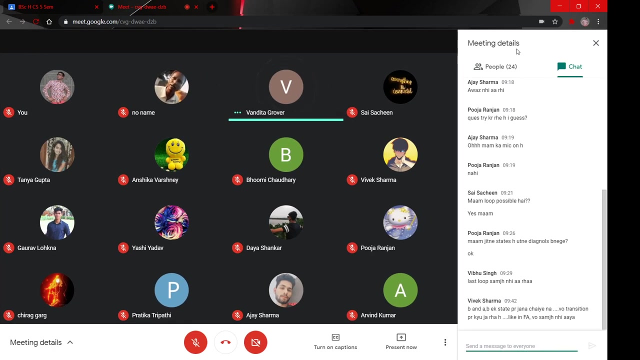 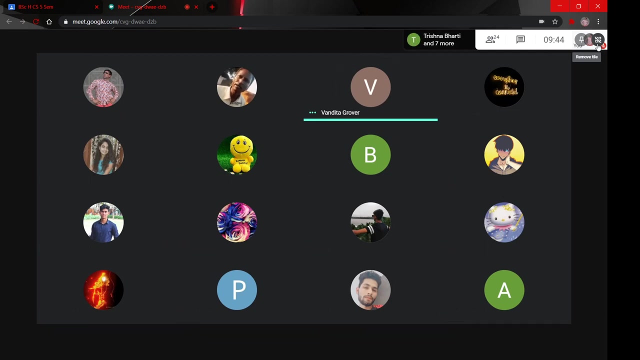 So pointers, tips, notes. Ma'am, the presentation has stopped. Yaar, it's okay, I will do it again. Such a waste of time. I think you should see it as a candidate. Please come again. It's not regrettable. 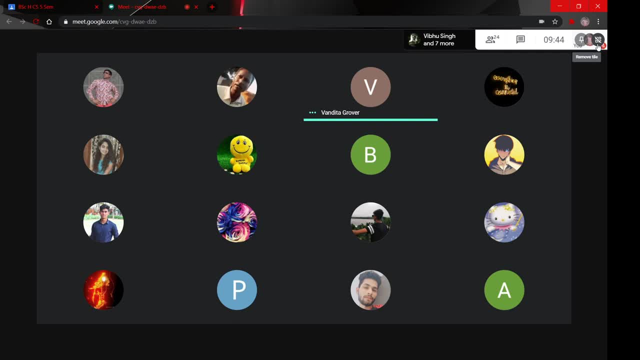 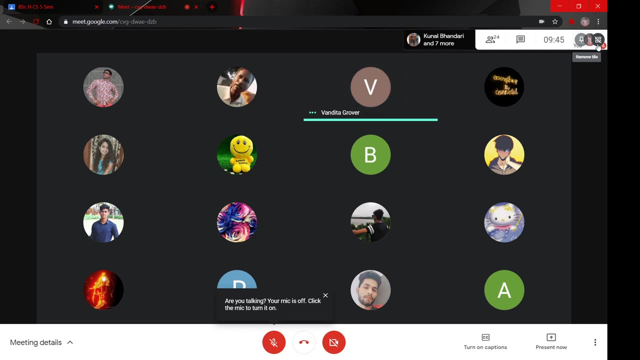 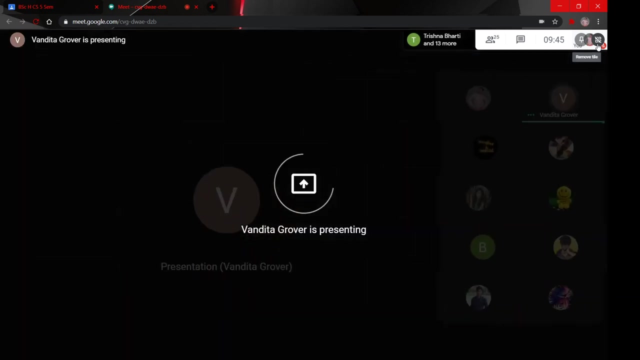 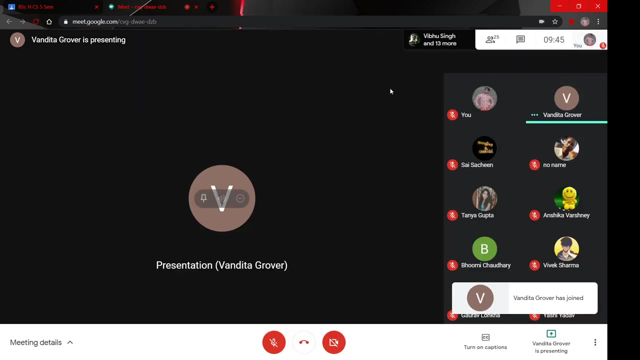 I said it that way. I don't know why I am pretending to agree. No, I think my first comment was worry. Yes, here, What response should I make to my application? Ah, Yes, okay, so this is my automata. is this visible? is this visible? 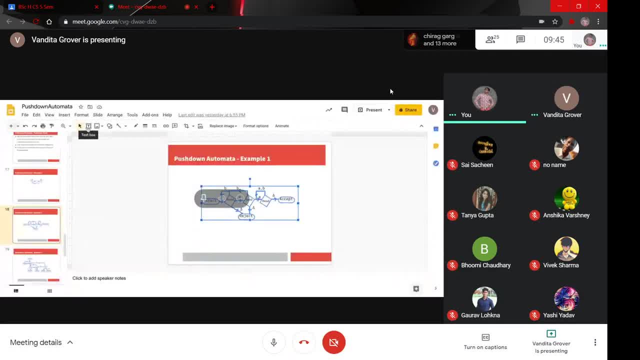 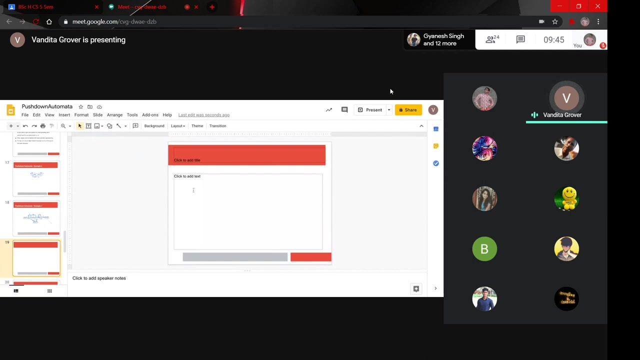 now what I am trying to say is he up need to even I. so what we are doing here is: you have created a state. yeah, I say stately, I'm gonna be school arrows, a joint girl, when suppose I enter an arrow over here, from here to here, and it's give us up. make our state when I 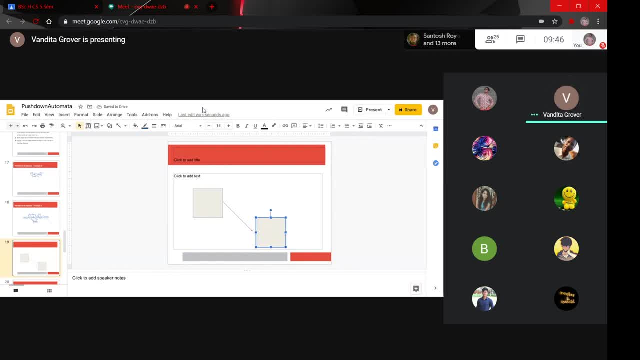 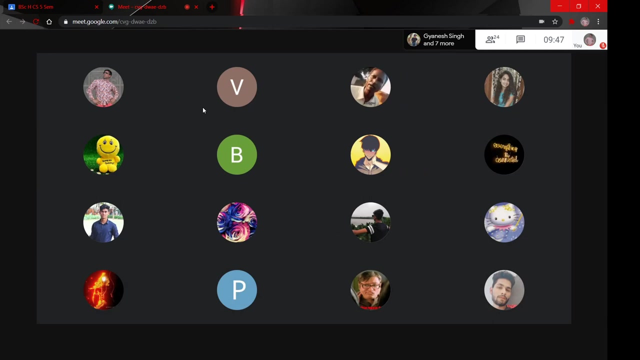 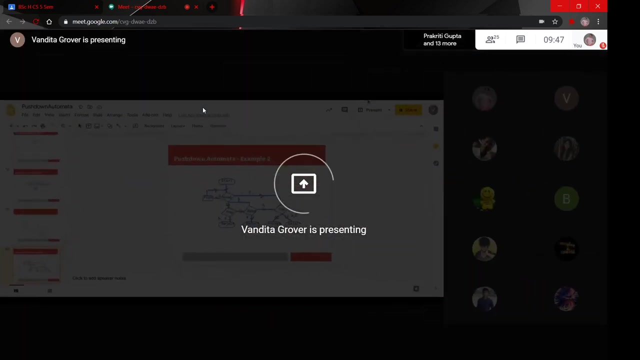 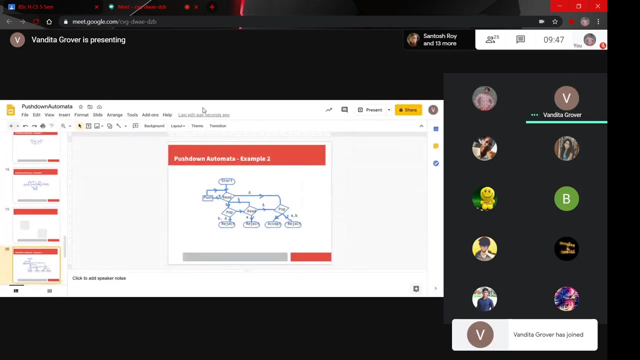 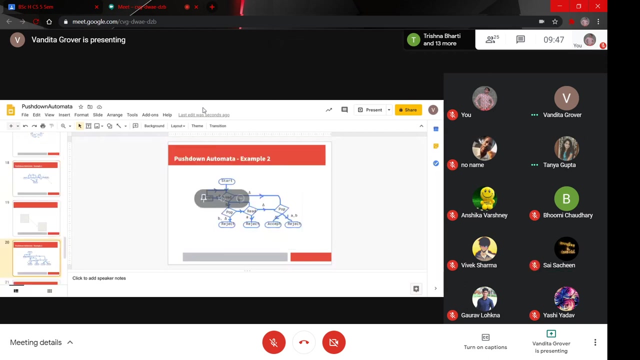 you, you, you, you, you seem extremely you, yes, mom. you, him, him, him, him. Just try to understand this one. I haven't come back to it, it's probably on the paper. There is one more question, but just try to see this question and understand what is happening. 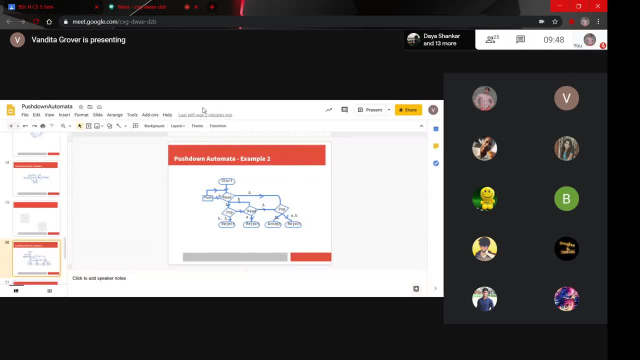 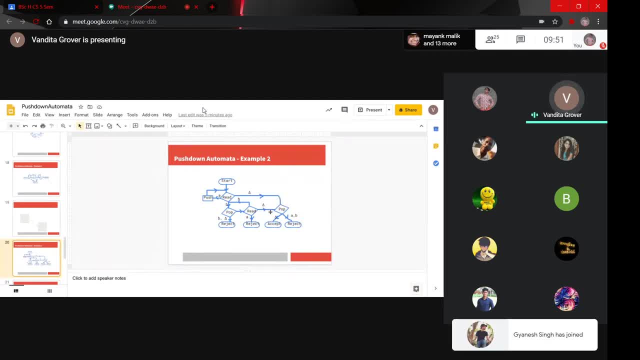 Agar mai yeh wala hai. It is just about connecting the arrows. Probably it is not connected correctly. If you look at this, whatever arrows we have, for example, the thread has an error read. If I call on this, 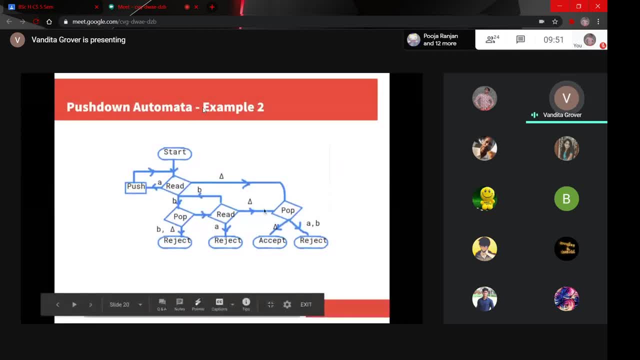 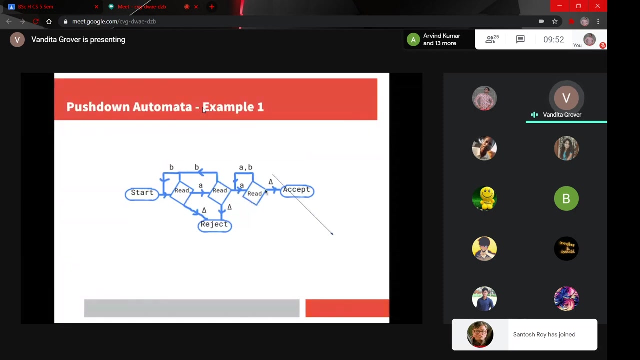 say. it's not that that particular edge is reading two different things. it is simply so. you could have simply done like this, all so. you could have simply done like this also, but this is a better way to represent. you could have simply done like this also, but this is a better way to represent. 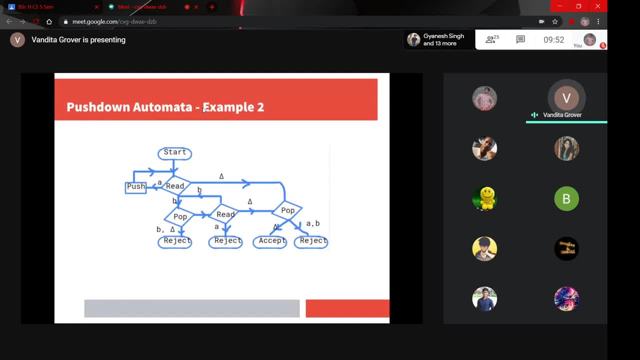 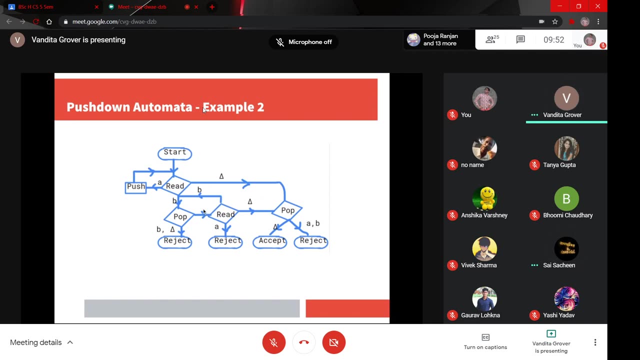 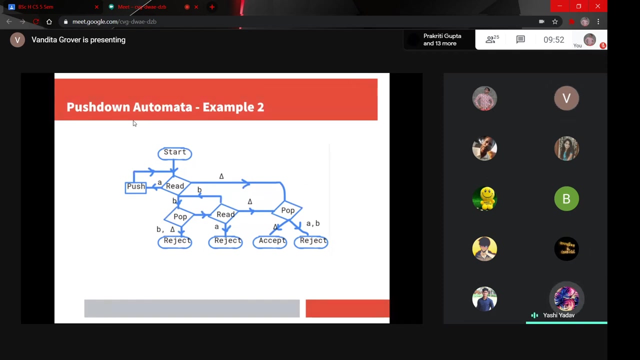 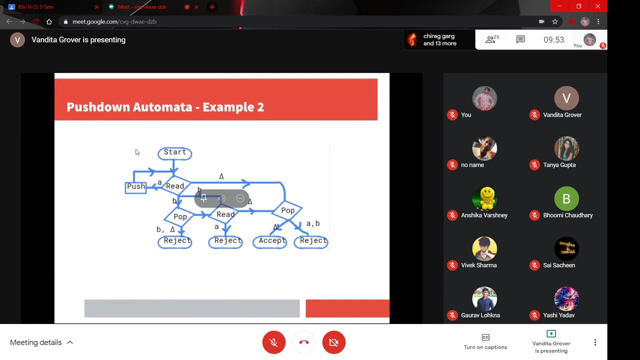 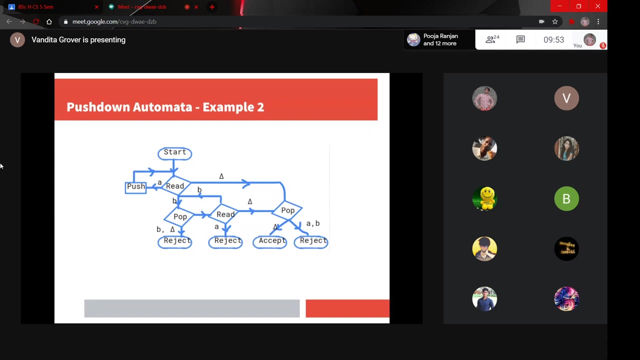 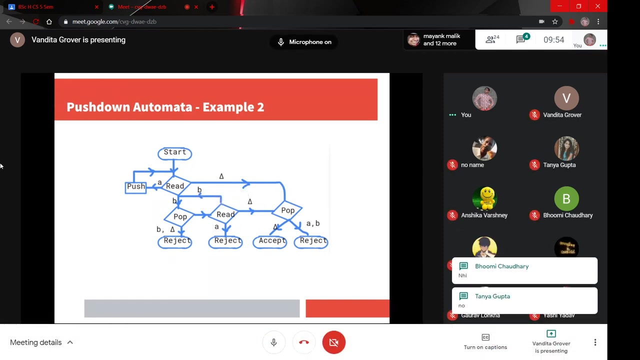 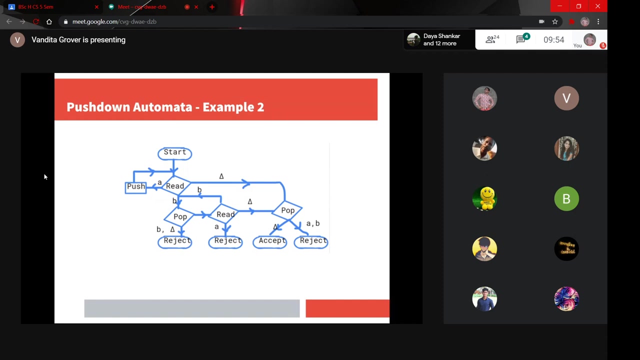 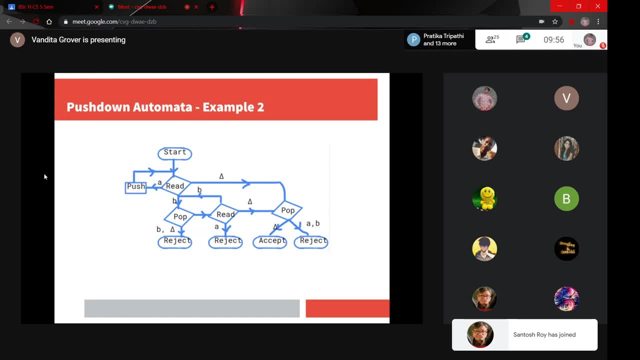 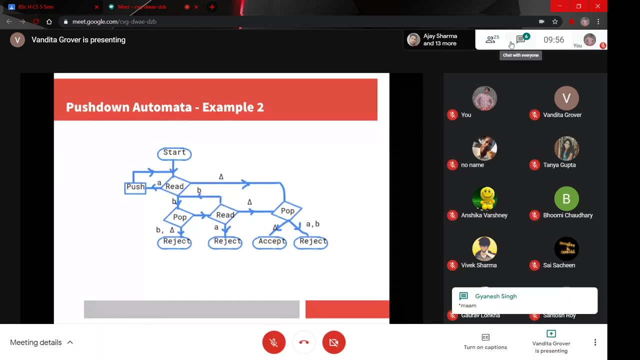 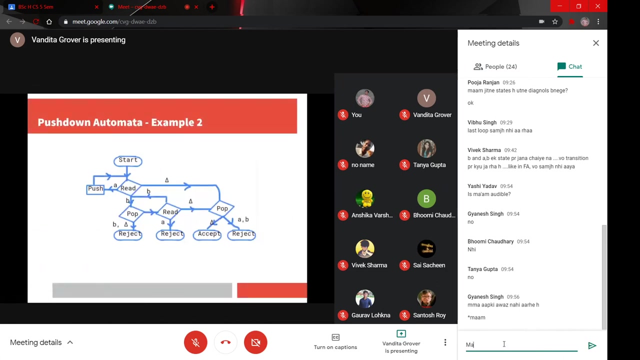 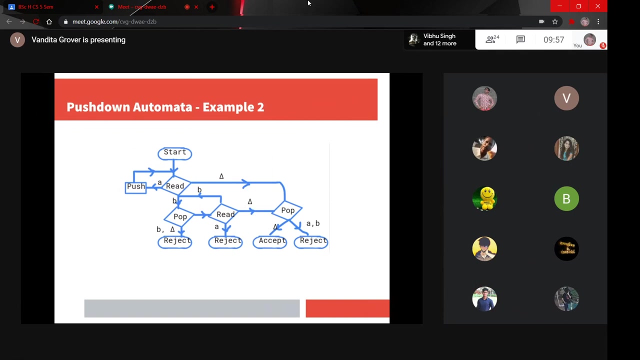 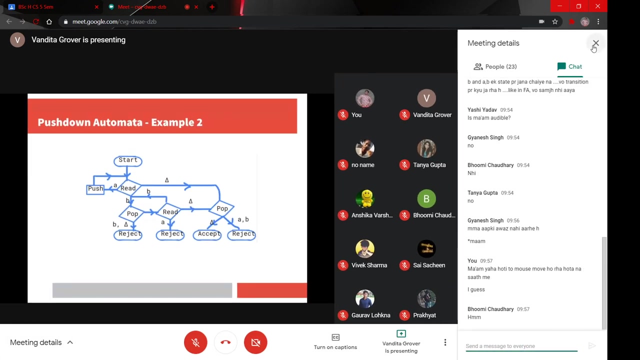 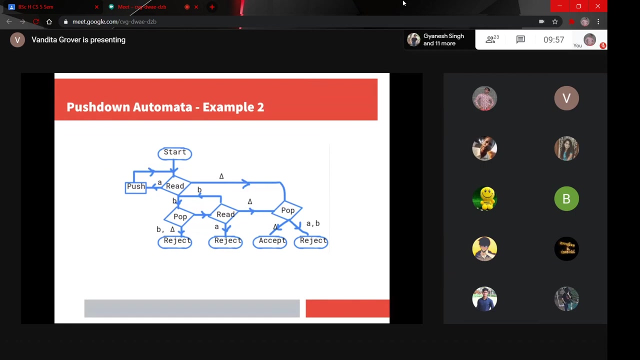 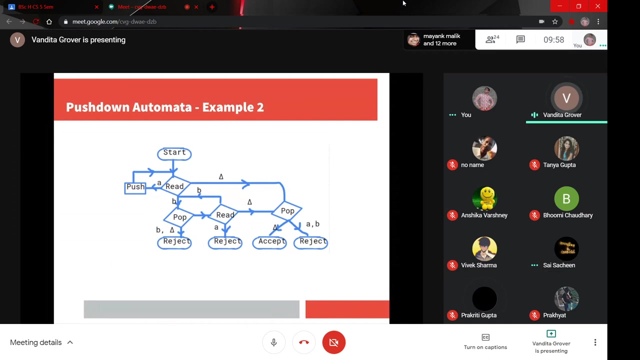 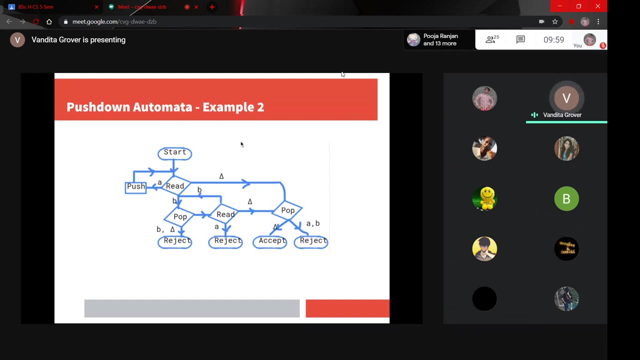 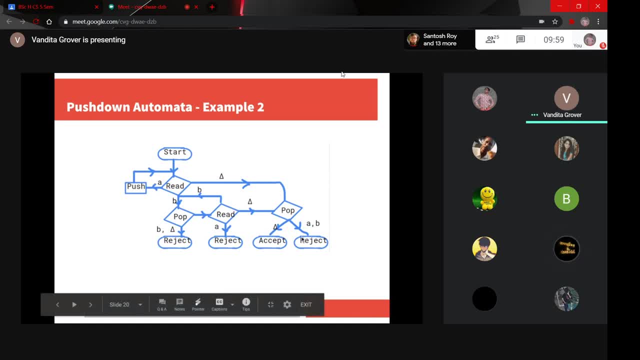 Let me get scenarios that blank what they're giving to knowledge: No as a baby therapy, or B A 2018 on a: A was pushed and A was left in the stack. Next time B came, What did you do when B came? 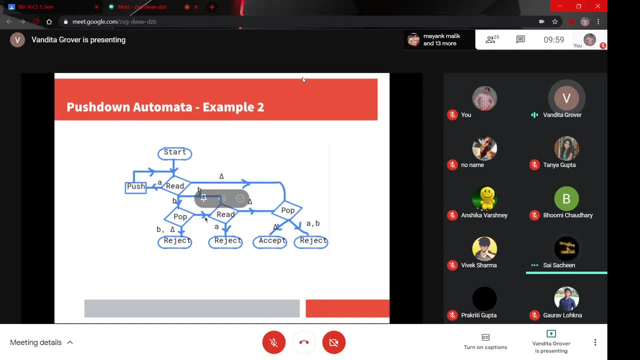 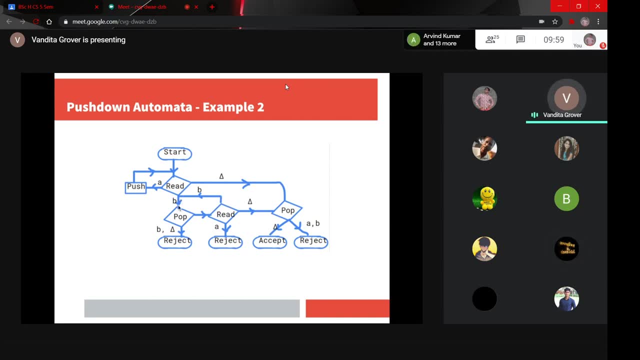 I popped, You popped and A was here. Yes, So you came to the read state. So you came to the read state. If you read B and popped, then your null will come. Yes, But if you assume that your null came after the pop, 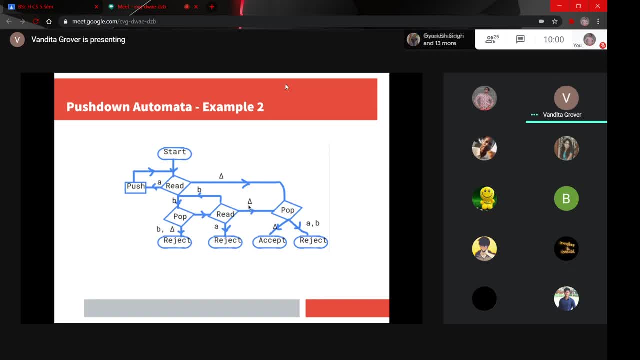 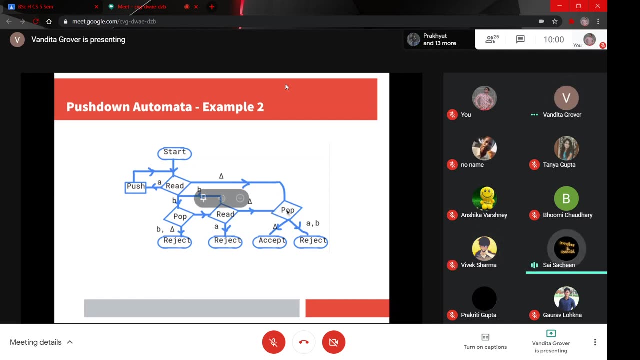 If A was there, then you read blank on the input type Yes. So you read blank and you popped. What did you pop? It was A. Nothing will happen for the pop. Nothing will happen for the pop. Once A was read, it popped. 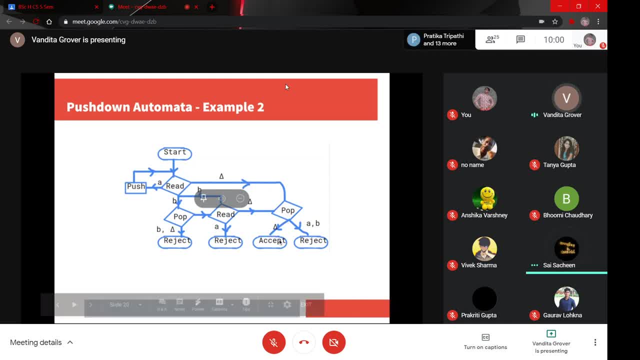 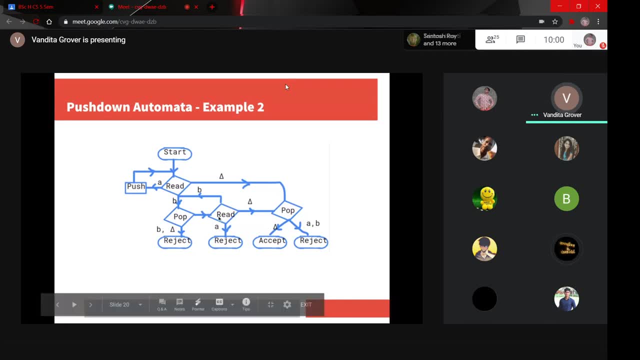 Then blank was left. Yes, Except A. If nothing will happen in the stack, then blank will pop every time. Now you take an input- A, A, A, B- And check for that, And I am not moving the mouse. 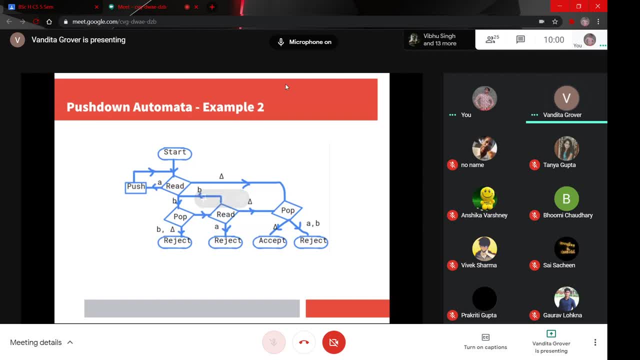 But I am not. There is some distraction today. That's why I am not going on mute. That's okay. It was coming. I rejected it. If it wants to come, it can come again. ________________________________________________________________ мире. 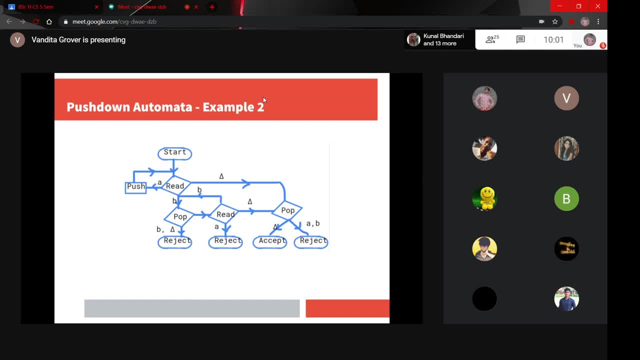 I want to move again And having only B, this writing is written the same, only I am not pulling the buttons for a while. The window should be drawn in that direction. Yes, Triplets Out Now do double A, triple B. 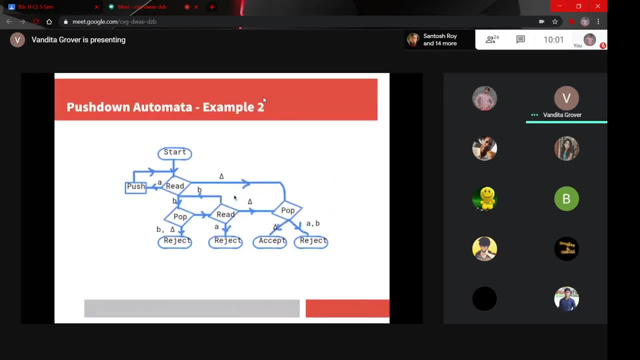 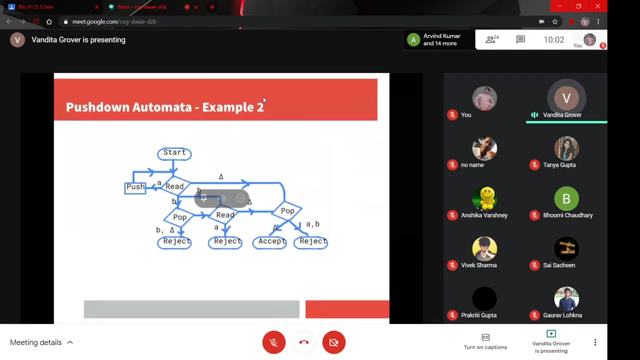 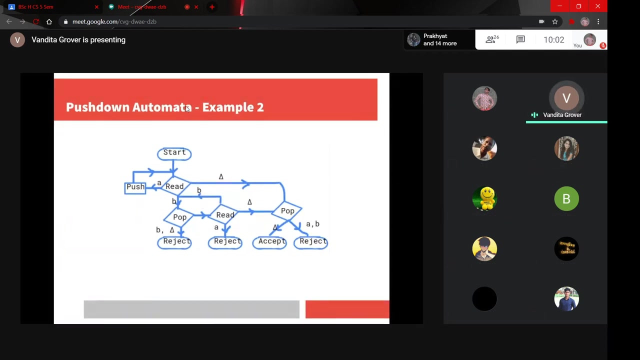 Do double A, triple B. I can't do it Now. do triple A, double B. Now do triple A, triple B. Okay, I'll show you how. I'll show you how to do this. The screen is visible, right? This is the input tape. 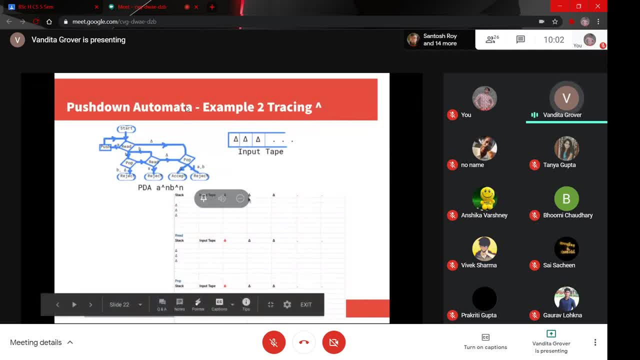 And you made a stack here and the input tape over here. You need to do same in exam Instructions are there in the stack Because you didn't add anything and there is blank on the input tape. Now you read it blank. read kiya jab blank. read kiya to aap: seetha pop mein, gaye pop kya hua, pop, hua. 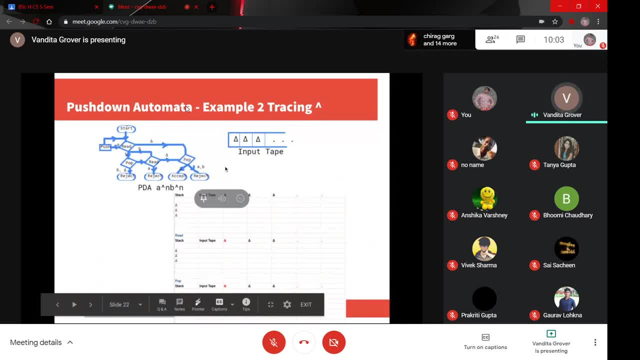 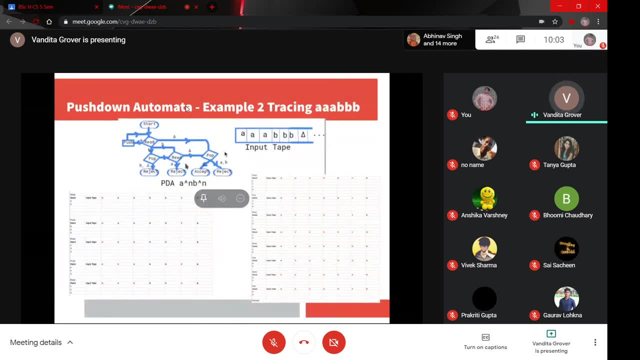 blank to blank hua to aap. accept. mein ho ho gaye matla blank. accept ho gaya hai to blank is a word in this language. now I will trace triple a, triple b, chike hai to input tape. 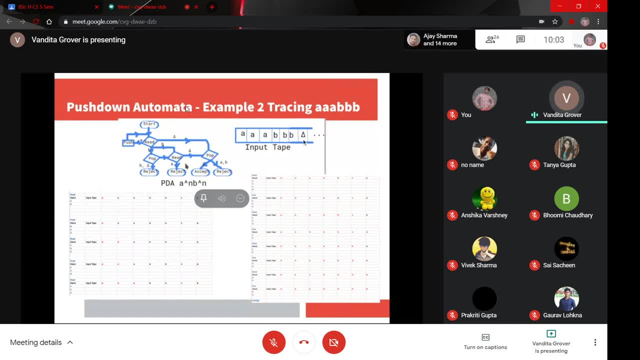 mein mere paas kya hai, triple a, triple b, aur jab string khatam ho jata hai to blank, to ab mere paas input aaya to main reed kiya. jab main reed kiya input tape se a. 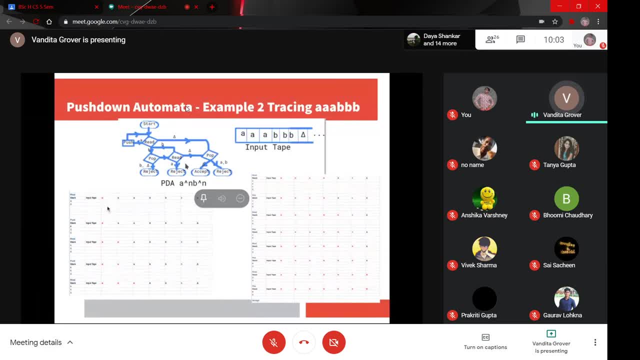 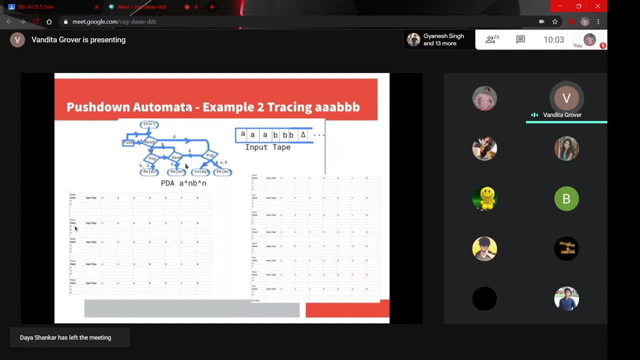 reed kiya ye mega website pe, ye thoda better dikh raha hai isko main reed karungi. a main cut off, kardia, jab main input a reed kiya to push me jayega, jab push me jayega. 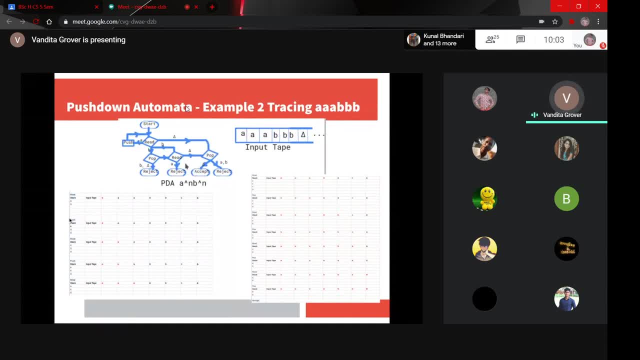 to stack mein a a jayega ye apko dikhana hoga exam mein, agar tracing dikhaga to to stack mein a a gaya. next time, jab stack mein a aya, mein wapas gaya main reed kiya. 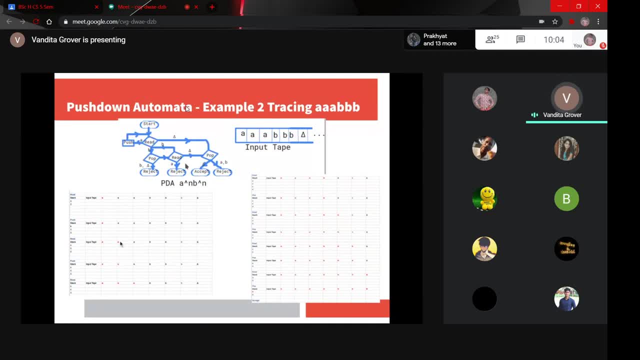 jab main reed kiya, to next wala input symbol read hua, wo bhi maine strike off kar gaya, ki maine read kar gaya, Ab wo push hua, Push hua, firse A push ho gaya. Next time, firse maine A read kiya, Usko knock off kiya aur stack mein push kar gaya, Ab maine stack mein 3 A's hai aur 3 A's yaha se hath gaye hai, aur maine dubara read mein chalegi. 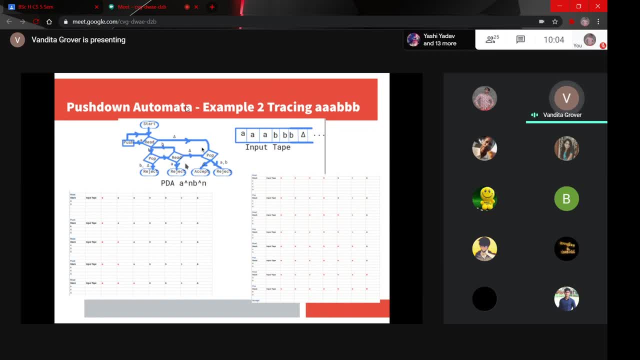 Is baar maine B read kiya. Jab maine B read kiya To jaise maine B read kar rahi ho to maine wapas nahi ja rahi, Maine pop pe ja rahi ho To maine stack ko pop karna shuru kala To pop. jab kiya to 1 A nikal gaya. Ab yaha pe dekho, I think dikhe gayi nahi, aap kushe. 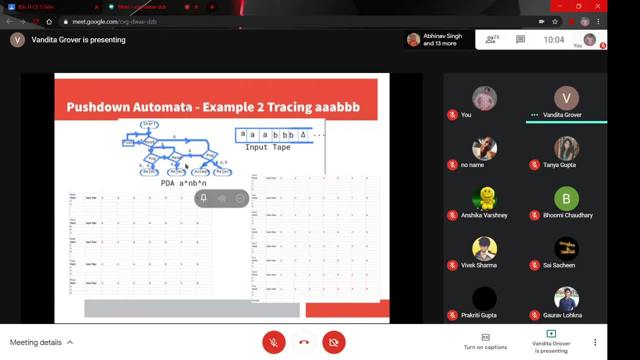 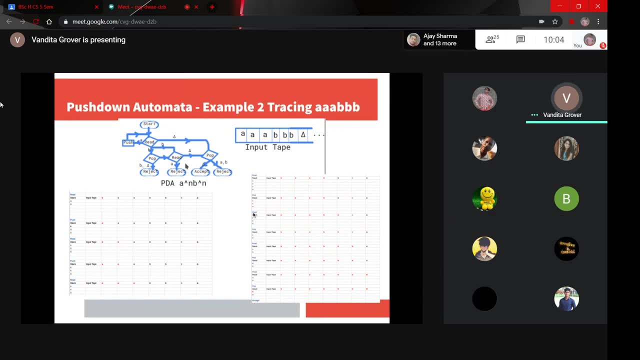 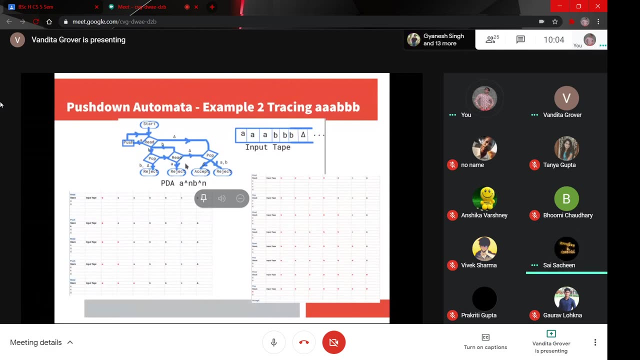 Zoom kare. Is there any way to zoom this? Dikh raha tumhe kya? No, ma'am, Bahut hi chota hai. Haan cheke To aapke paas. aapne jaise B read kiya to aapne ek cheez pop kari, Lekin top pe gaya tha ya 3 A the to pop kara to 1 A hath gaya. Uske baad aapne firse read kiya: 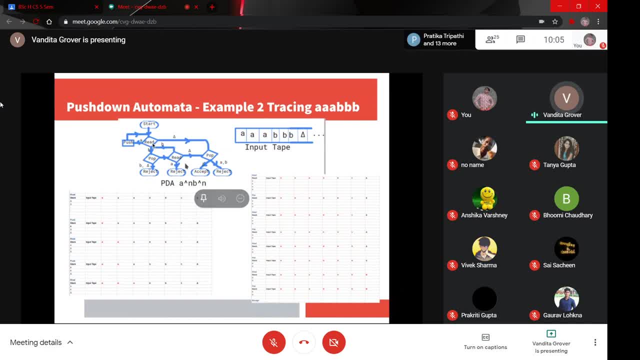 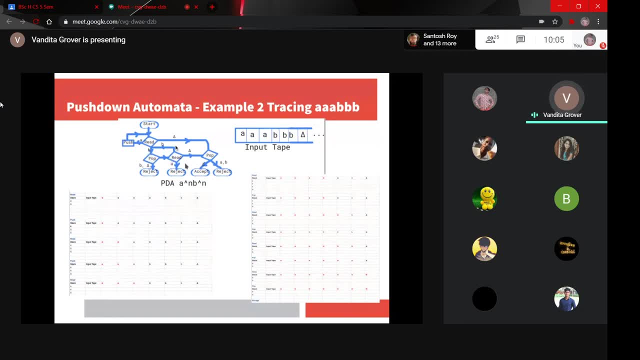 Pop karne gaya. firse read mein gaye. Agar B read hota hai To, agar B read hota hai To aap. dekho, this is not a confusion, Tanya. Is read se gaye to bhi yaha pe aayenge. aur is read se gaye. 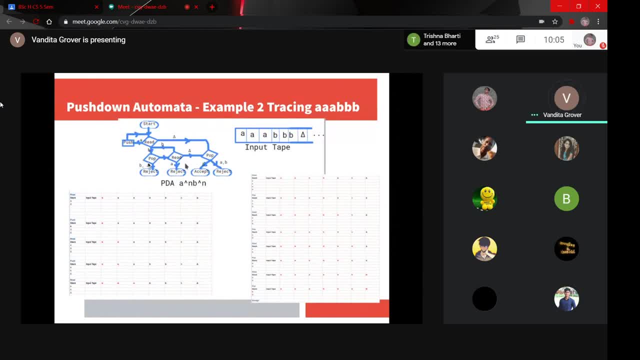 To bhi yaha pe aayenge. I am just joining the two arrows. Fir aapne pop kiya, firse aapka ek A read hua, Ek A read hua, aur agar A aaya tha, Yaha pe A hona chahi. 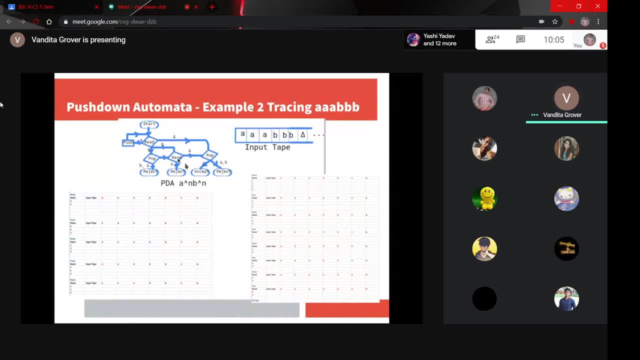 Yaha, mujhe A likhna chahi, Agar ek A pop hua, Fir main read me gayi, Fir 3 B ko read kar diya, 3 B ko read kar diya To mere paas main firse pop me gayi aur 3 A ko pop out kar diya. 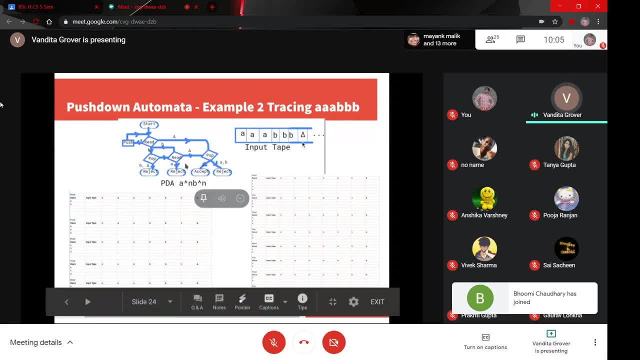 Next time mera symbol hai blank Tape pe To jab blank hai to maine firse stack ko pop kiya Mere stack me a blank kiya To mere stack me a blank bacha hua tha To mere string accept ho gaya. 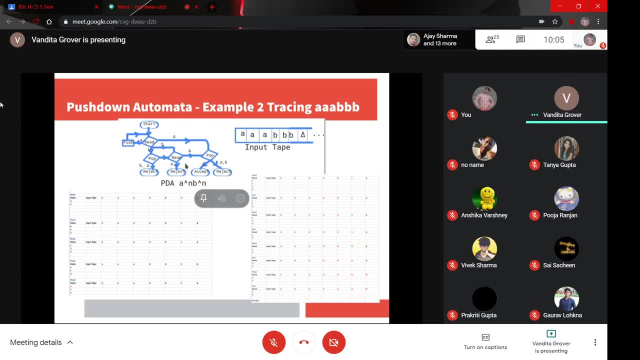 Cheek hai pen aur paper se karoge to hoega Ma'am, jo third word bhiya tha aapne triple A, double B, wo bhi accept nahi ho ga, Aur agar ma bolu double A, triple B nahi ho raha. 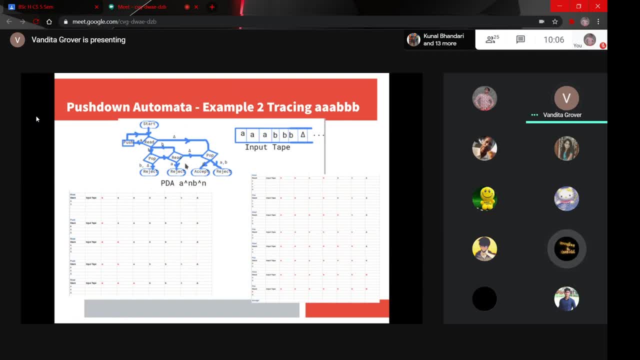 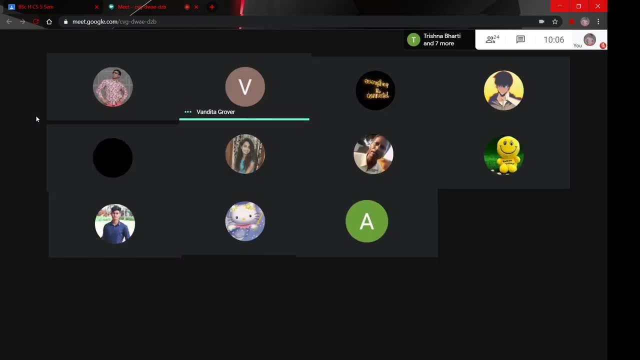 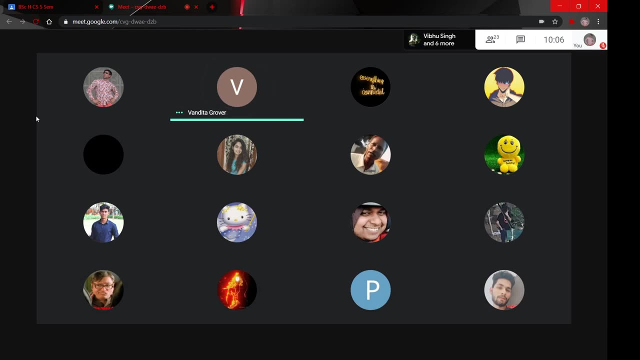 Agar ma bolu A B, A, B ho raha, A, B, A, B. True, A B. Is A, B, A, B being accepted. No, ma'am, wo pehle rejet ho jayega. Second day aate rejet ho raha hai, To agla bhi rejet karne ko option hi nahi hara. 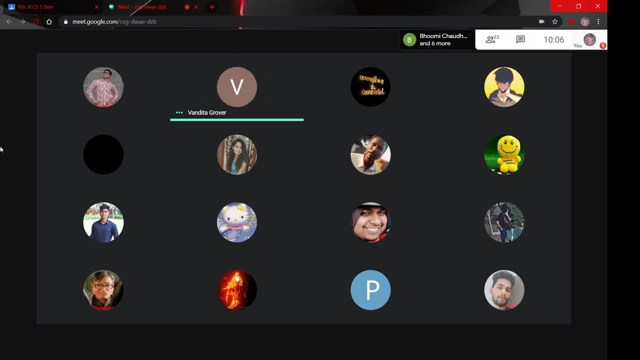 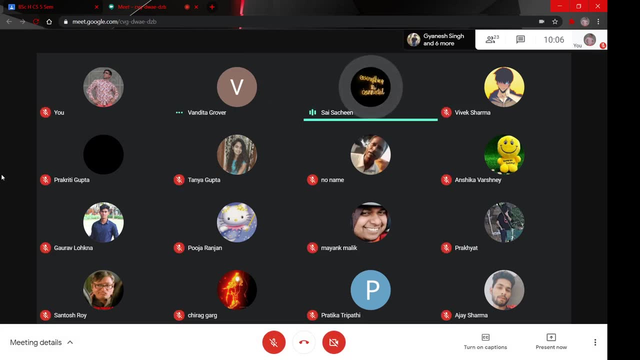 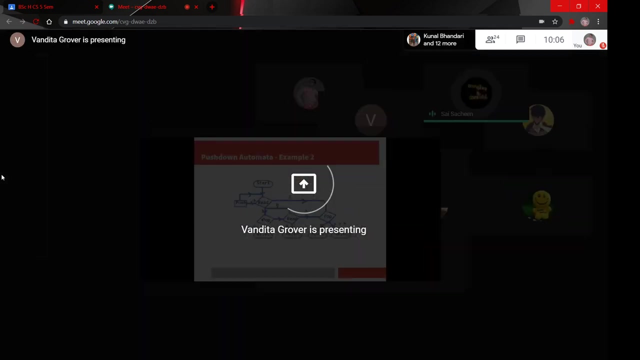 To what is the language of this finite automata? What is it accepting, Ma'am? equal number of A's and equal number of B's, And B's are always after A's Matlab. starting. A se hoge, aur phir B's aayenge, aur equal number me hoge. 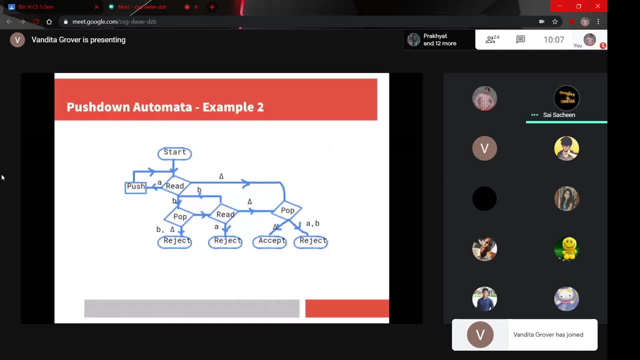 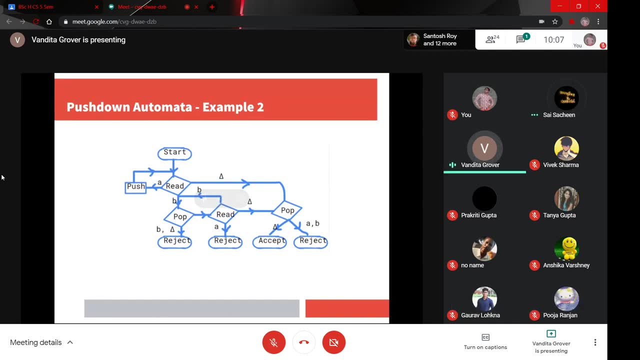 To yeh kaunsi language hai A and B and mo Matlab A and B and regular nahi thi na Nahi, ma'am Aise nahi accept karwa para tha usko, Lekin kuch kaun automata me aapne stack add kiya. 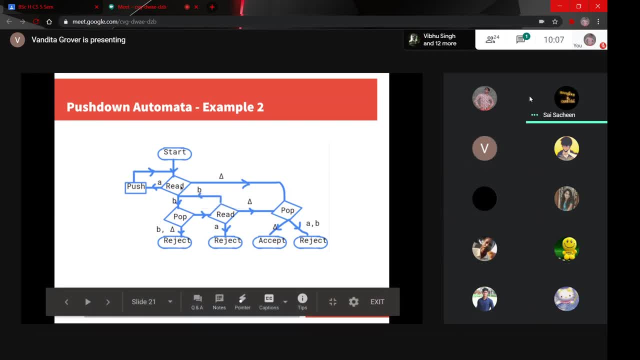 Aapne kya kiya. Aapne har B ke aapne stack add kiya. Aapne har B ke aapne stack add kiya. Har B ke aapne paherle ek A rakha hai. 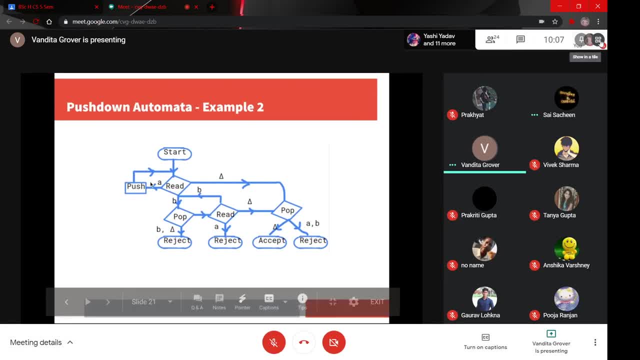 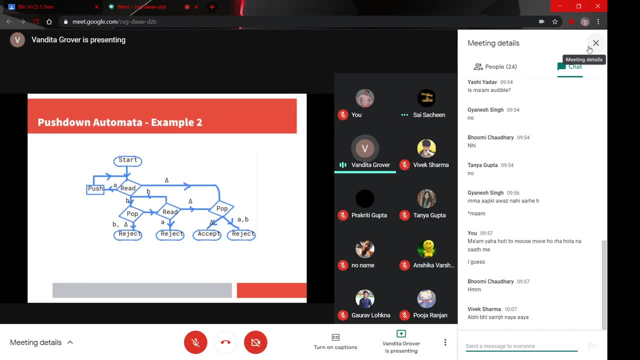 To aapne un A's ko stack mein dal ke remember kar liya. You wanted to match the number of B's with number of A's. You could not do it in finite automata. Soki finite automata ko yaad nahi rata usne kitne A padhe to. 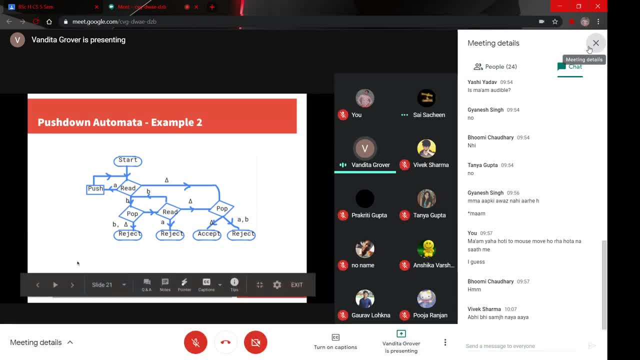 PDA to itne yaad hai, kuki usne stack mein dal gaya. the To usne yaad rakh liya, Jab usne yaad rakh liye to aapne agni paar, jab B padhne sharuh hai to. 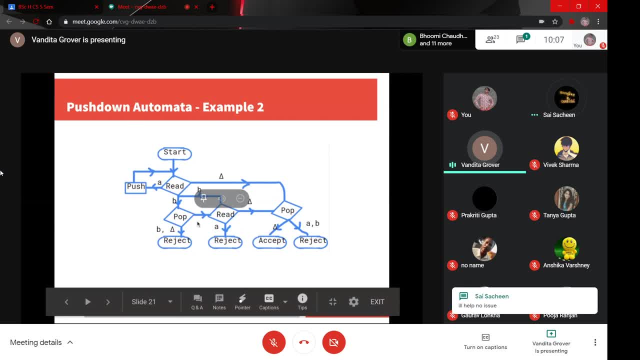 har B ke liye ek A aap pop kar raha reho, Har B ke liye a pop kar raha reho and match kar reho. So equal number hi aega. Agar uske alawa kuch aur aata hai, toh aap reject koi. 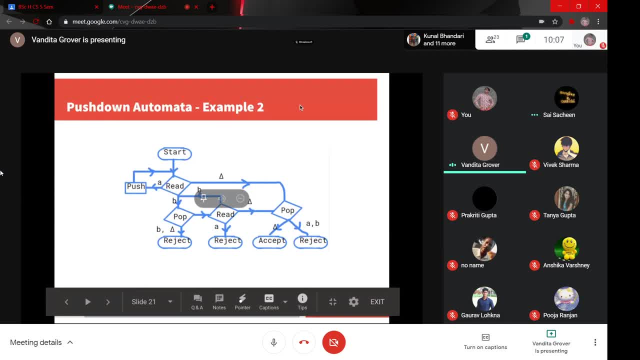 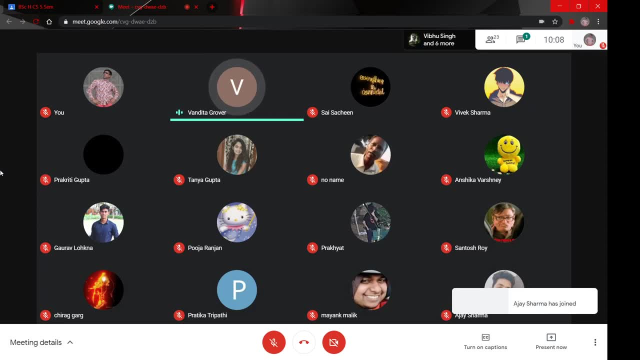 Yes, So this is a language A and B, So I wanted to cover these two examples only. Please try these examples at home and then try for palindrome. also Palindrome, try karo. or reverse string. reverse karo, Yeah, I think. reverse hoi jayega. 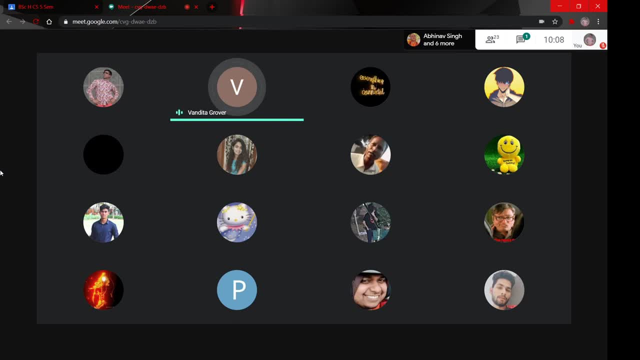 Palindrome. try karo, Try for a palindrome and try building an automata for palindrome. Kal mein test dungi pumping lemma ka Time bache ga toh palindrome ki baat karenge, ne toh friday ko karnege. 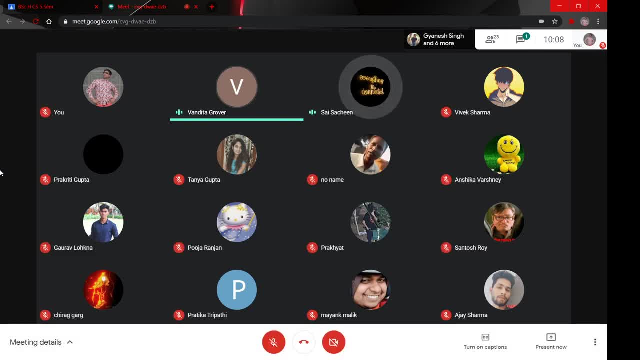 Chik hai. Okay, Ma'am, palindrome ke liye pehle usse pushdown automata ham banaye, usse baat try karenge. Okay, so there are two things. Agar aap regular language accept karwa rahe ho, kyunki wo finite automata bhi accept karte ho. 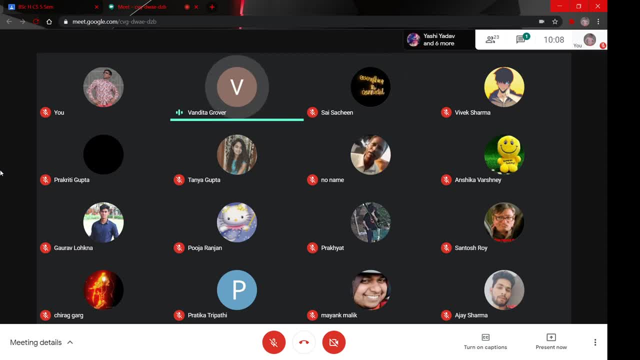 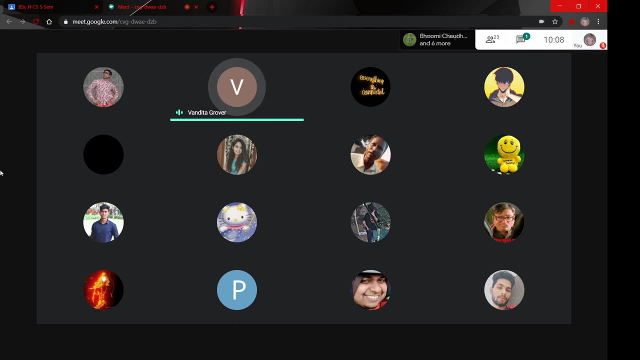 finite automata me memory nahi hoti, So most likely Aapko stack ki zaruvat nahi padegi. if you are making a pushdown automata for regular languages But non-regular language jab banawge, toh us case me aapko most likely pushdown automata ki stack ki zaruvat padegi. 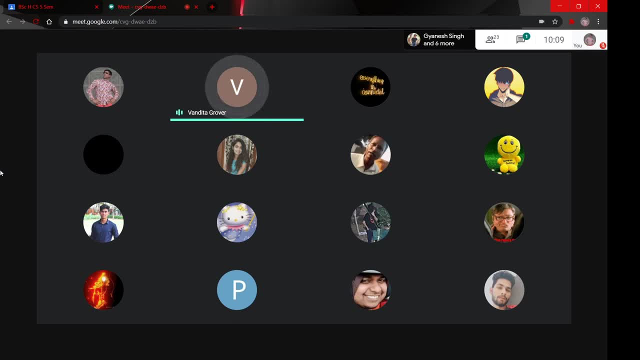 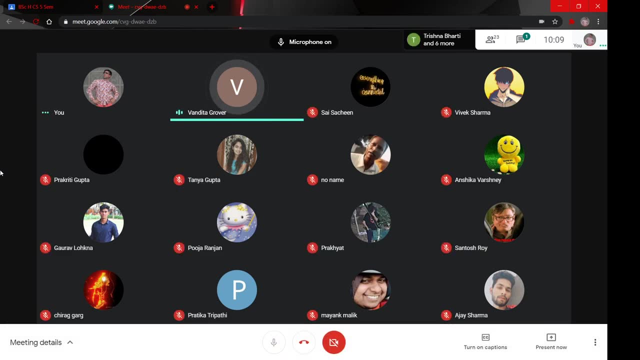 kuch na kuch remember karne ke liye. So you have to see the question to. basically, you have to think how you are going to do it. Vivek kaha nahi samajhaya, batao Kya samajhaya. 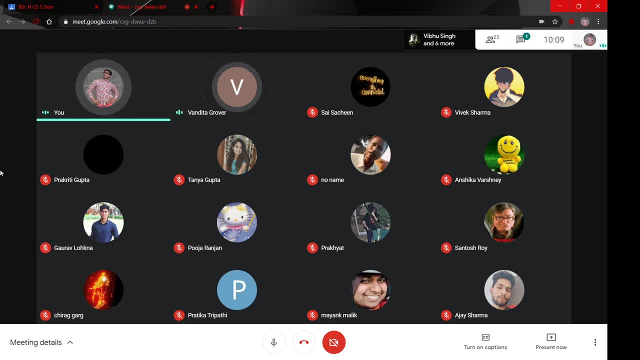 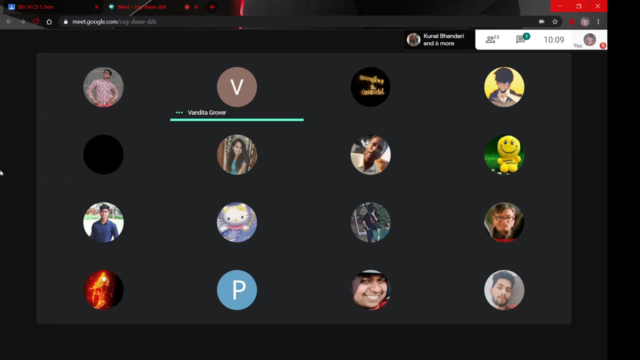 You understand. Okay, Vivek, mein ek baar aur aapko batar lagat yun Buye. You must tend to make sure they hear you, Vai, What's a tall wei yahing gel, say du.